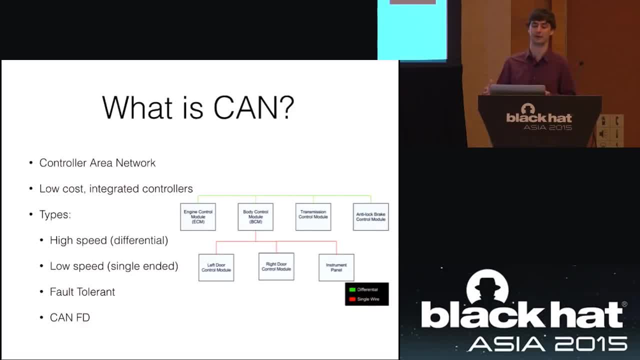 higher. It's single-ended Ground is actually the chassis of the car, so you just need to run one wire out And you'll see this in your light control, door control, radio- things that are less critical than just more convenience features. Fault-tolerant CAN is what you'll. 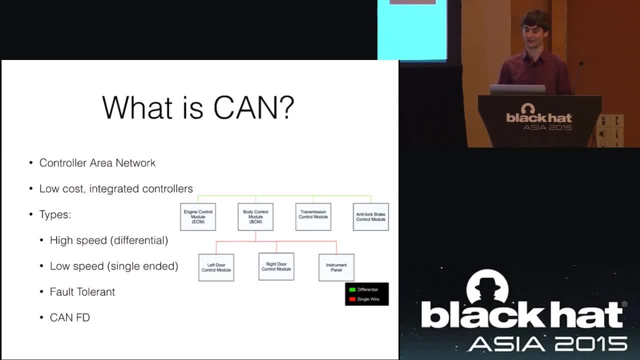 often see in airbags. This is actually a pretty neat trick. What they do is it's high-speed CAN, but if you cut one of the wires it becomes low-speed CAN, So it's got some tolerance there. The new thing is CAN FD for flexible data, which nobody uses yet, but it gets around. 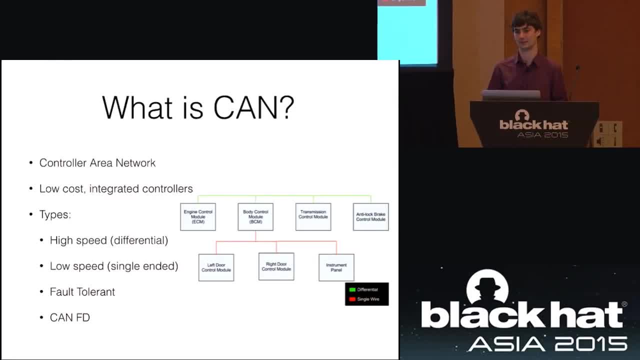 some of the limitations right now of the size of the CAN message. It's probably going to make its way into cars in the next. I don't know, knowing how fast the automotive industry moves- five years or something. And what does this look like in a car? Well, there's a little. 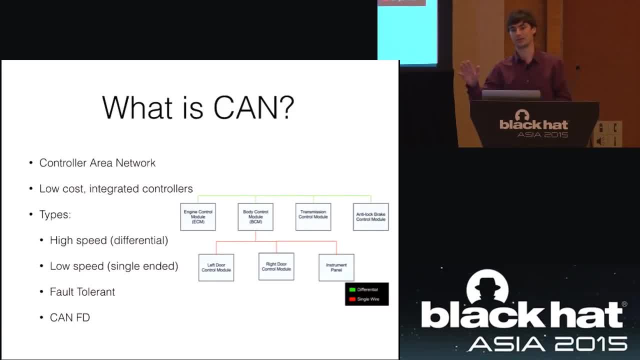 diagram over here which hopefully is legible, and it's just showing that you have often a bunch of CAN buses. This is a bit of a simplified example. You have four controllers on a high-speed bus in green, So these are your more critical. 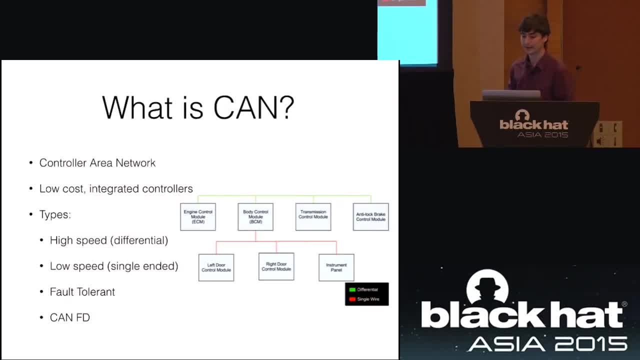 controllers. You've got an engine transmission, anti-lock brakes as well as your body control module. That body control module is then connected to the low-speed bus shown in red, which is connected to some things like door controllers. Yes, there's a controller in most of the doors. 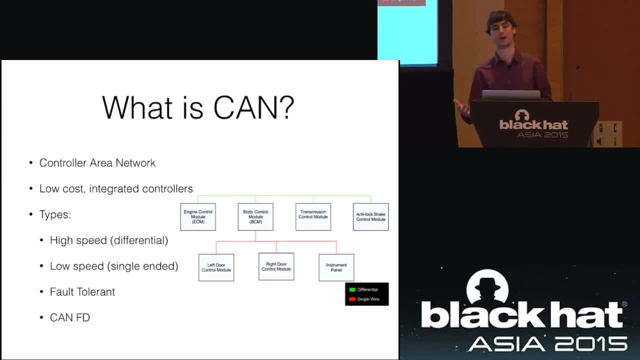 in the car nowadays Also an instrument panel that reads out your speed and engine RPM controllers. now in pretty much everything in a car, They're just giant computers, to the point where, if you have automatic seats that move back and forth electronically. 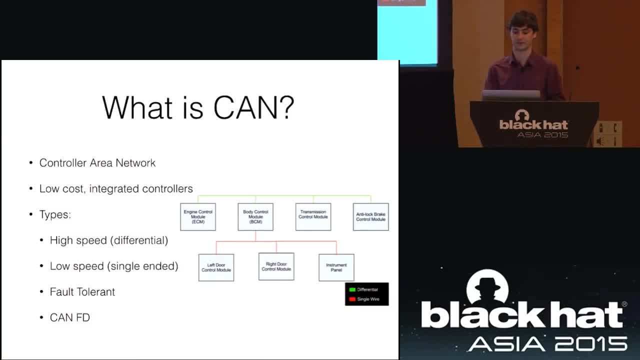 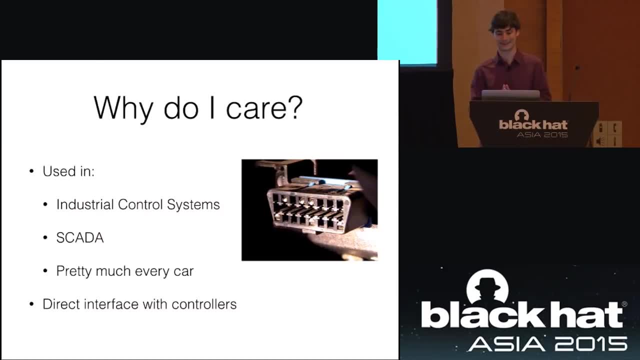 that probably has a microcontroller that's likely hooked up to a CAN bus or something similar. So why might you care? Hopefully you're interested in this stuff or you wouldn't have come here, but in case you have no idea, CAN is used. 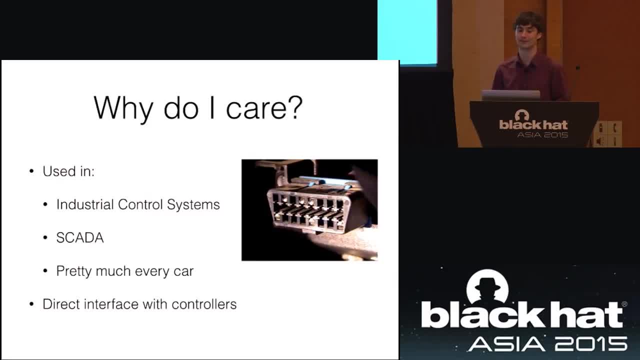 a lot in industrial control systems. It's used a lot in SCADA systems. You'll see it just sort of all over the place in industrial because it's pretty good at being reliable in terms of there's like a CRC built into the actual hardware level. 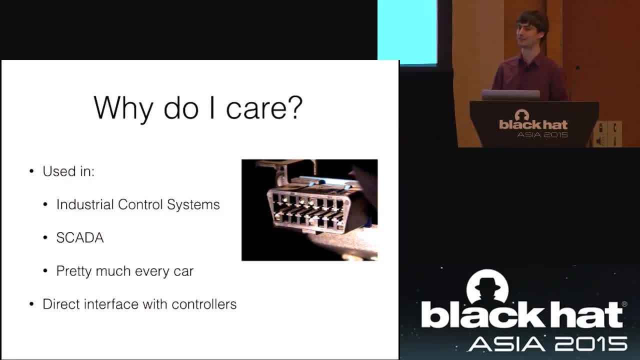 protocol and it also has acknowledgment built in, so guaranteed message delivery, all this stuff that industrial people like. But it's also in pretty much every car, And what I mean by that is every car after 2008 sold in California and, sorry, sold in the US- had to have CAN. 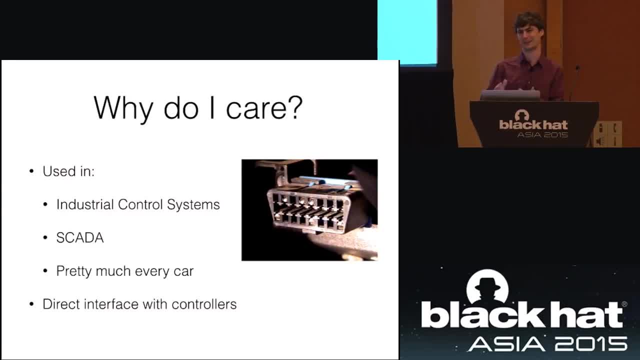 So all of those and everything after 2005, had to have CAN In 2005,. it starts to phase its way in some as early as, like the early 2000s. Mercedes was sort of the first to use it. 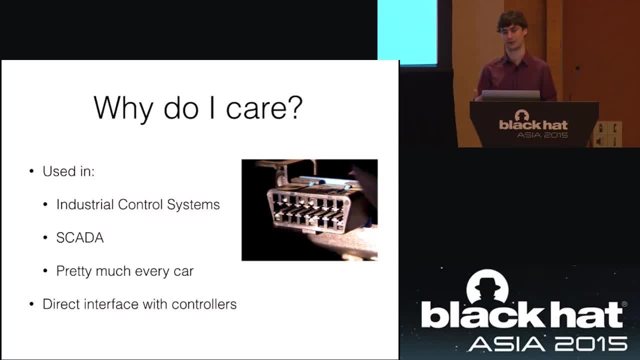 And it's a direct interface with these controllers. So often you're talking well, when you're using this, you're talking actually directly with code that's running on an embedded controller that is also responsible for things like operating your engine or unlocking your doors. 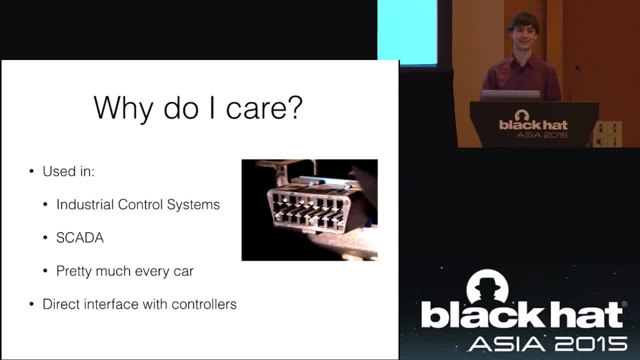 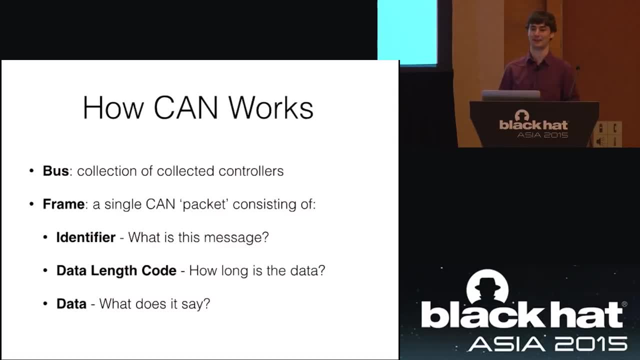 So clearly there's some potential to do some interesting things. So how CAN works? we're just going to define some terms here. First one is a bus. I've already said this a few times: Basically just a bunch of controllers connected together by CAN. 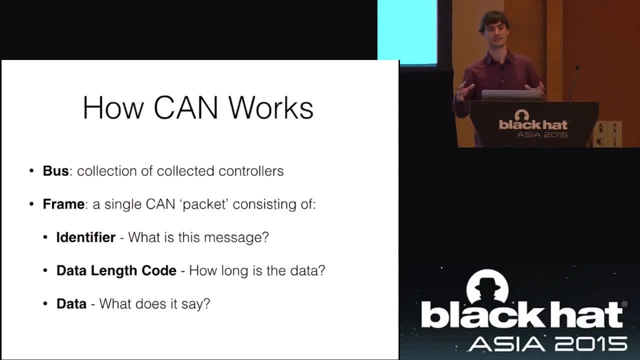 It's a CAN bus, Great. A CAN frame is sort of a single data packet, It's sort of an atomic thing that you can send out on this bus, And every frame will have an identifier, a data length, code and data. 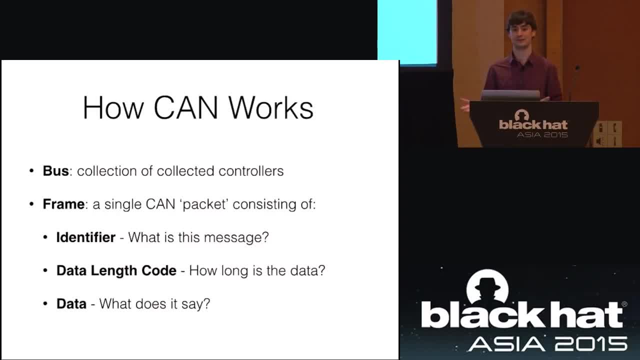 So the identifier is just very simply: what is this message, What does it mean? The data length code, how long is the message, How many bytes? And, finally, the data is the actual data And if you draw it out, it looks a little bit like this: 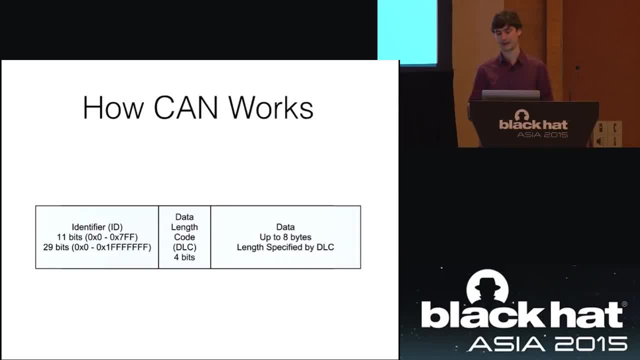 Identifier is either 11 or 29 bits, usually 11.. Data length code is just a 4-bit number, And then you have your data And that's really all there is to CAN is an identifier, a data length and some data. 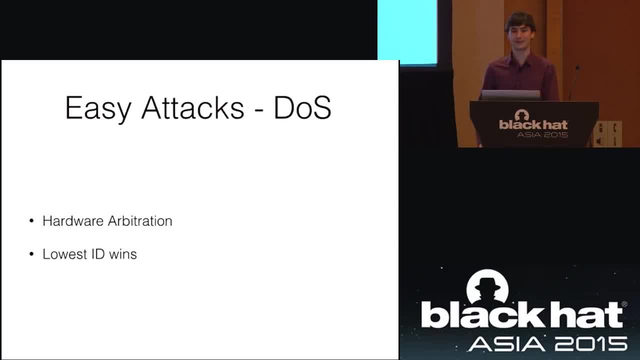 And it's as simple as that. So let's start with the super easy attack- that is so easy it's almost not worth mentioning, but it's sort of entertaining, So I'll mention it anyway- Which is a denial of service, The way that arbitration works in CAN. so whenever people want, 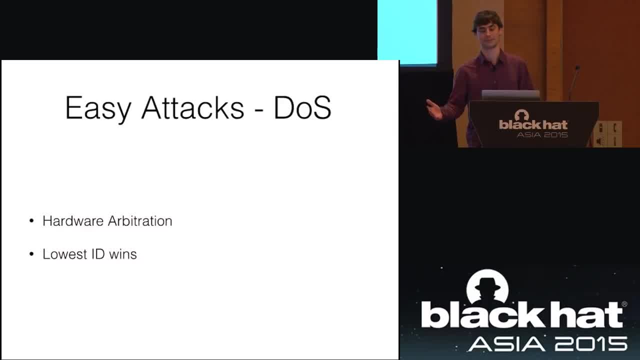 to talk on the bus. everyone sends out their identifier And while they're doing this they're also listening to see what identifier is being sent. So if I'm sending message 500, I'll start putting that out on the bus, But if I see a lower CAN ID then I will shut up and go. 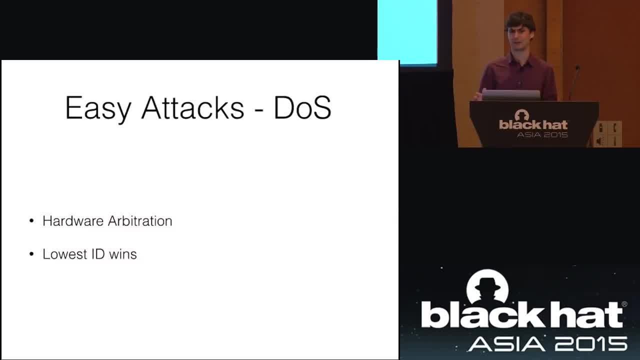 into listen mode. I won't get into how the electrical part of this works, but basically the lowest ID always wins and gets control of the bus. Now what's fun about this is that you can come up with a very easy proof of concept for denial of service, which is: 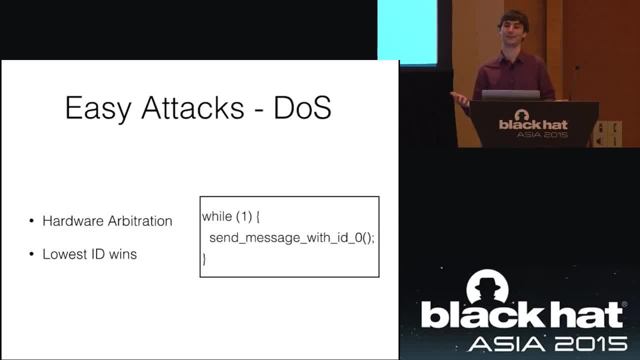 just keep sending a message with ID 0. And if you do this, nobody else can really talk, Because they get to the arbitration. you send 0, everyone else goes into listen mode. Then they get to the next arbitration phase- you send 0,. 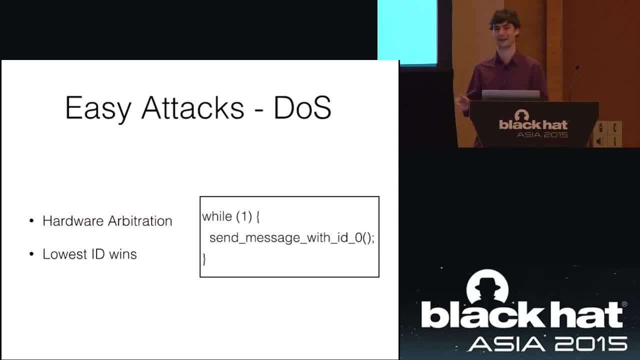 and this keeps happening And this is really simple stuff. but it actually will do some not so nice things in a car. It depends on the vehicle, It depends on what CAN bus you're on. But I did this. Actually it was a company I was working at. 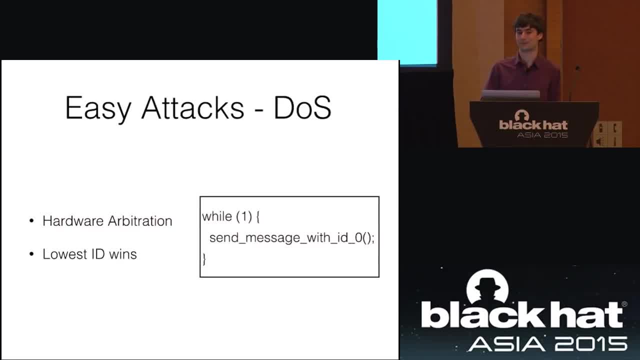 It was. the CEO of the company had a Chevrolet Volt And we were playing around with it And I plugged into it And I didn't realize that the tool I had was sending messages when I plugged into it And I think the actual message was ID 4, not 0. 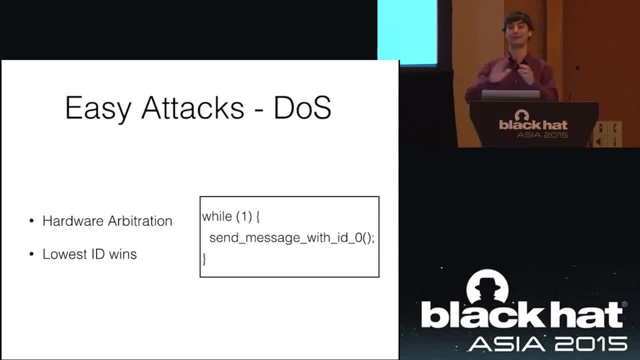 But it was low enough, And so what ended up happening was every fault code and every light turned on all across the dashboard, lightened up like crazy. But it was a Volt And the Volt actually has some great fault codes. It doesn't just have your service. stable track service. 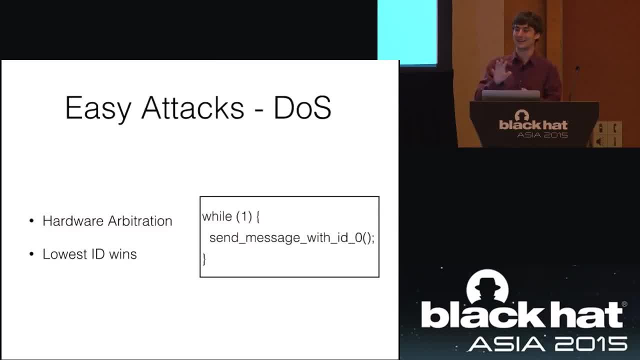 power, brake service, power steering, all that stuff. That all came up. But then it comes up with because the Volt's a hybrid engine not available, which is actually my favorite thing. I've seen a car say other than the next line, which is: 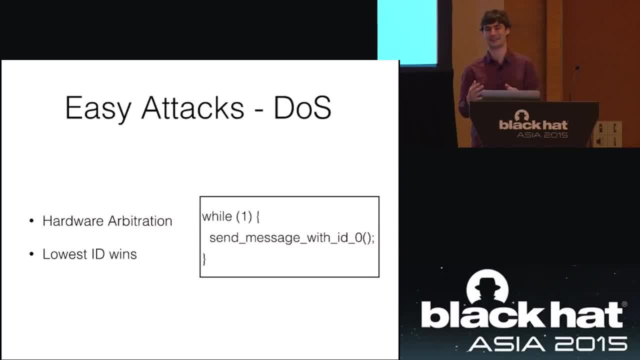 service soon. So if you lose your engine in a Volt, they're expecting you to get to the service station before you run out of battery, I guess. But that was sort of a fun message. I've never seen anyone recommend that. I you know. 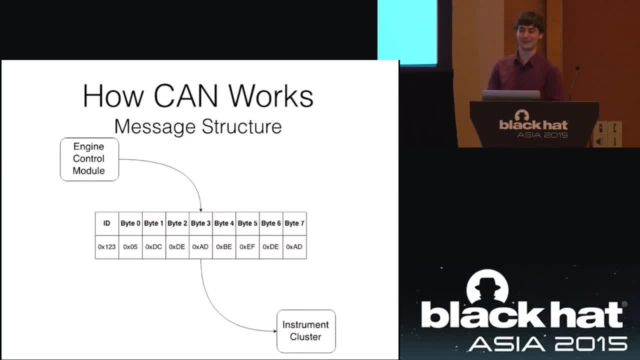 it's just the engine, It won't be that bad. So let's take a look at sort of how messages move around on CAN. So we have an engine control module in this somewhat contrived example, But this is really how it works. 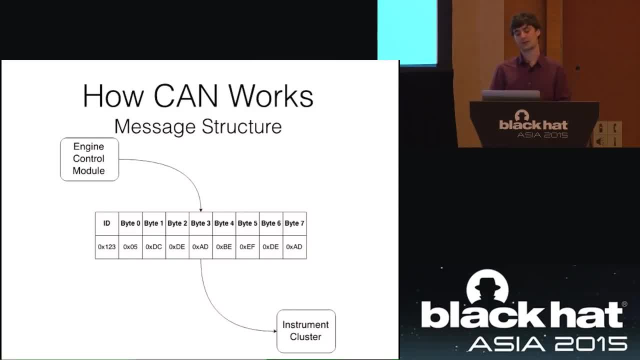 I've just changed the numbers. Engine control module will send a frame And it will be received by everybody on the bus. In this case, we are going to send it or receive it with an instrument cluster, And what I mean by instrument cluster is that panel of gauges. 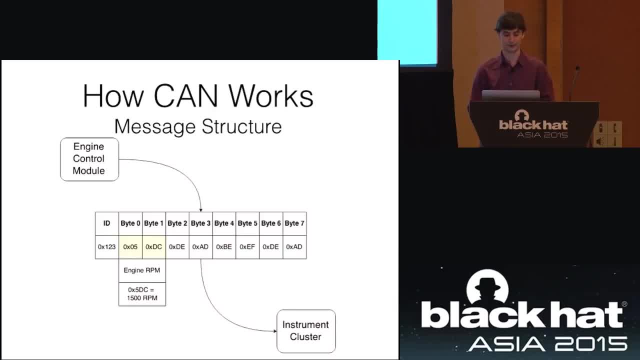 that you look at while you're driving, And in this case, we're going to send it to the bus. And in this case, we're going to send it to the bus. In this example, we are going to decode the first two bytes as: 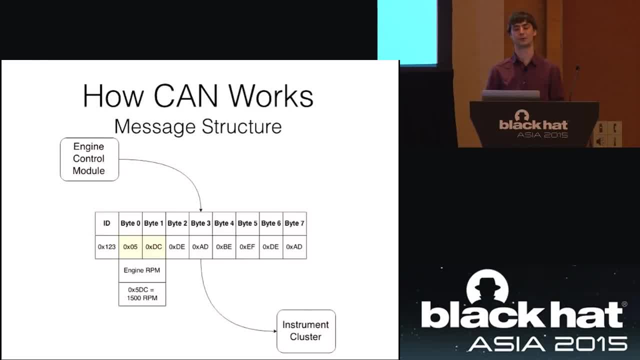 the engine RPM. How do we know that? Well, we have to agree on all of this beforehand. Nothing tells you what any of the bytes mean in this message, other than you create a database, called a CAN database, of all these messages And you program that into every controller on the bus. 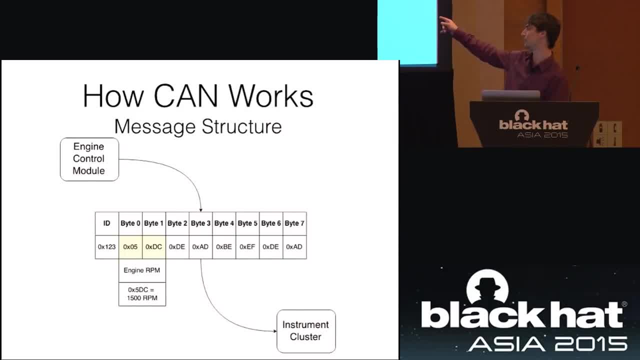 And now those controllers are able to say: oh, this is message with ID hex123.. And I know that the first bytes, that's engine RPM in that endianness And often they'll be like a multiplication factor or maybe an offset. 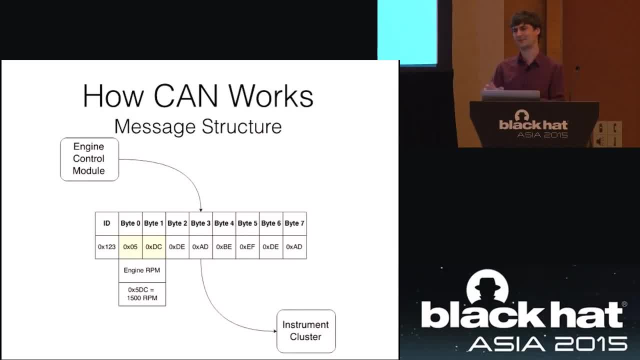 You've got to add or subtract something to get to real value. But then eventually you do a little bit of math And it actually has real world units. So in this example I just assumed, OK, we'll just multiply by 1, don't add anything. 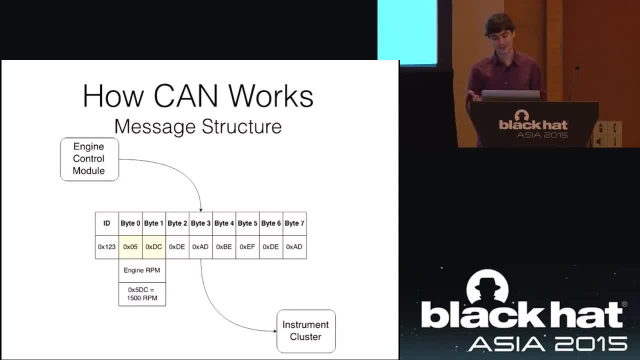 And we just get OK. 5 DC is 1,500 RPM. It might be a little bit more complicated in a real vehicle, But it's just a multiplication factor and an offset And once that's done we're going to send it to the bus. 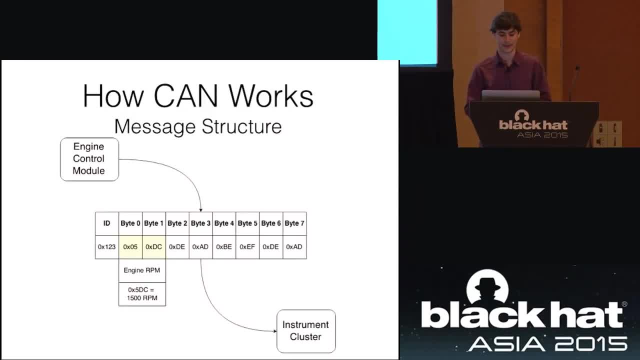 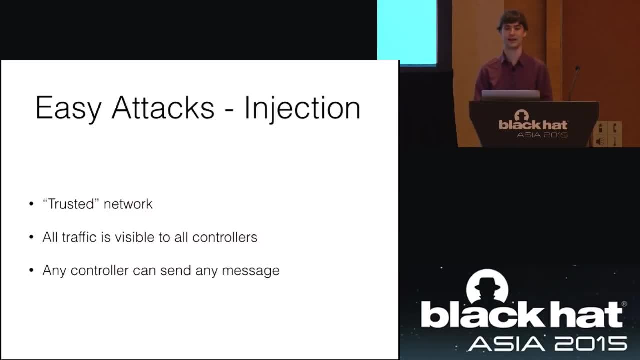 And once that's sent out it can be received by the instrument cluster which can display it. So this brings us to another really pretty easy attack to do. that follows really naturally from that which is injection. We sort of talked about how CAN bus all these controllers? 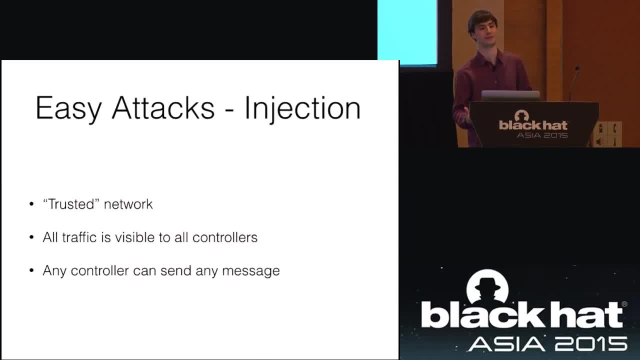 are just connected to it. There's no routing or anything. So everyone sees every message And everyone can send a message with any ID. There's no limitations. There's no MAC addresses or anything, It's just identifiers. So it's sort of a trick. 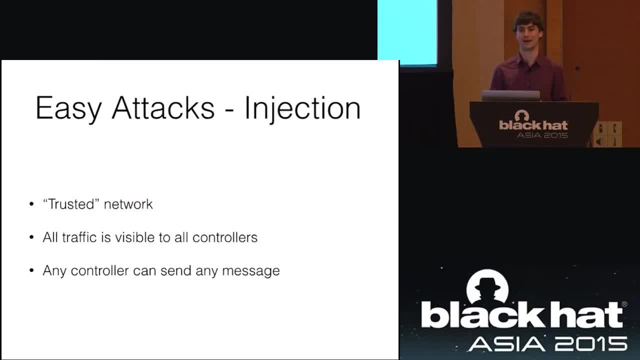 It's a trick. It's a trusted network. They're expecting you to not put anything bad on it. That's sort of the assumption. So this means that we can do something simple like this: We take a rogue controller. Now I say rogue controller. 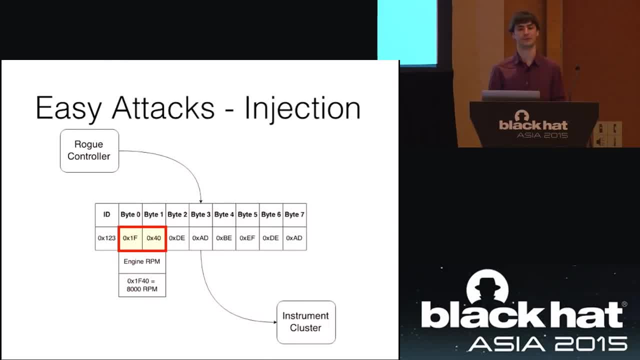 It could be a tool you plug in manually, But it could also be if you found some vulnerability in a radio or in the telematics system or anything else that's on the car that connects to the internet. And remember, Nowadays We're connecting more and more cars to the internet. 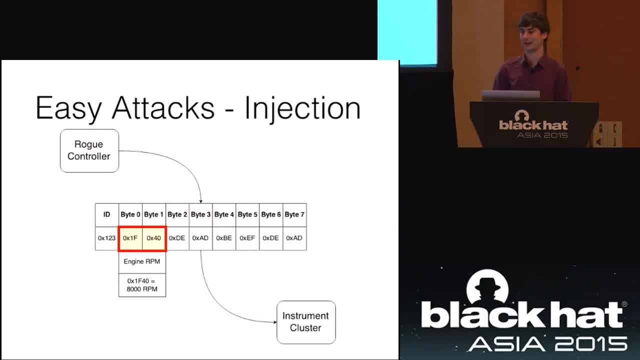 Or it connects over some other RF link. That's potential for one way to get in, But once you have control of anything on the CAN bus, you can do stuff like this And we could just send a different engine: RPM. What happens when we do that? 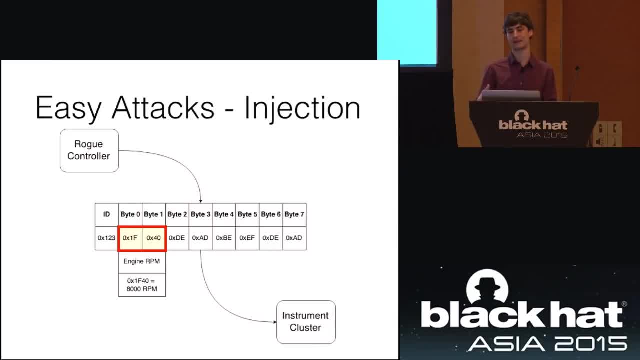 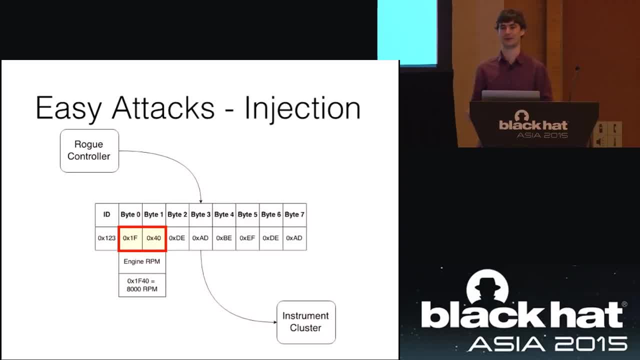 And whenever one has the most zeros in it, they're going to get sent out at the same time, That value will win. So if somebody sends zero and the other person sends all ones, the value received will be zero. But if you send it faster than the real controller, that's. 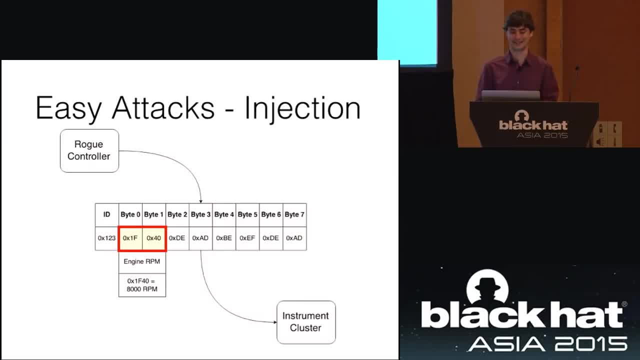 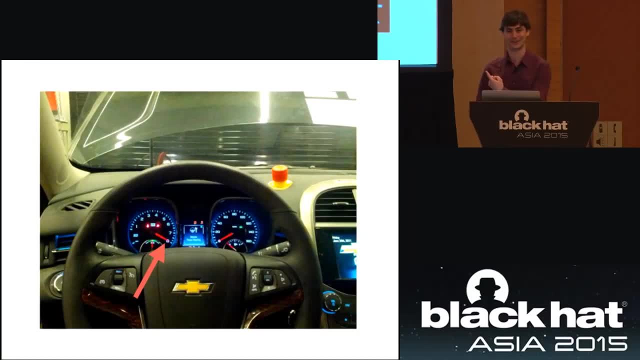 supposed to send it. you can usually just take over and really mess up operation. So if you do this on a car, you get that This car actually has no engine in it. We're just sending a message And, as you can see, it's like: OK, 8,000 RPM. 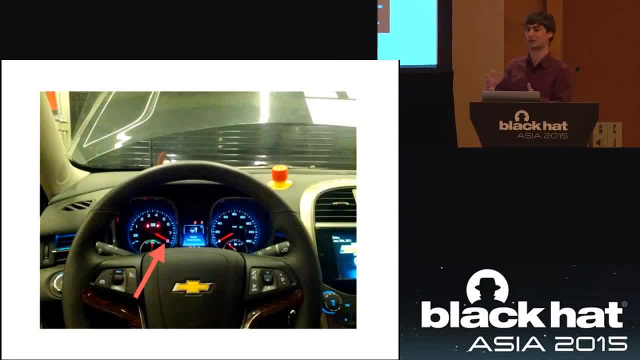 That's fun. This is a bit of a benign example. It's just a really easy example. It's easy example to see. But remember that cars, there's so many controllers and they're making so many decisions based on this data. 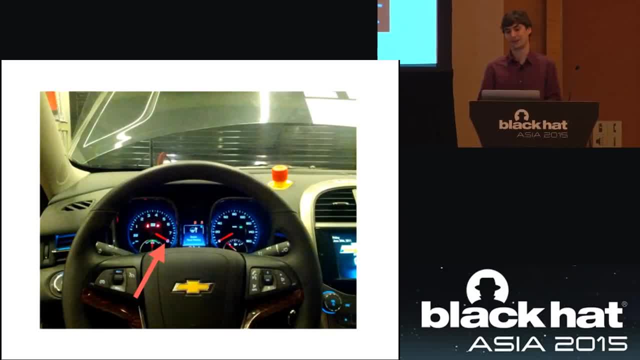 So if you can tell a vehicle, hey, here's some fake data that makes you think, oh, an accelerometer is reading a very high value. that might be like a crash situation. that could potentially have a chain of effect. Cars do certain things in crash situations. 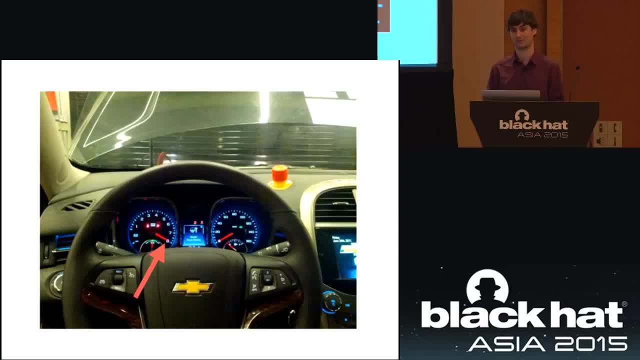 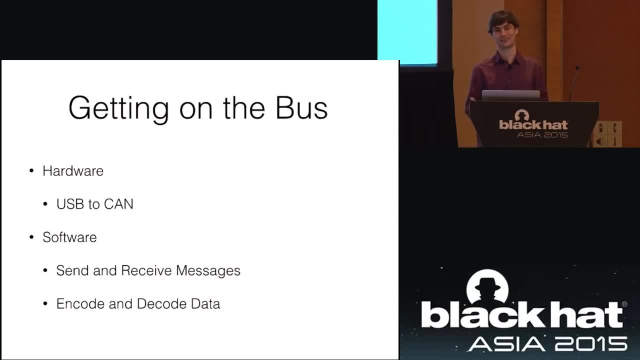 They do certain things in different operating modes And you can fake these things out. So how do you get on a CAN bus? We talked a little bit about two pretty simple ways of sending stuff, But we need to actually be able to send messages. 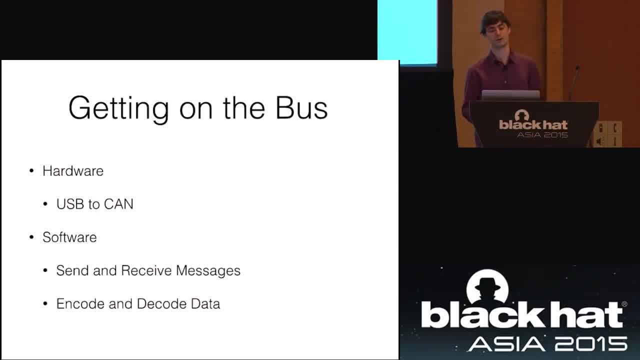 And the answer is you'll need some hardware and some software. Most computers won't talk CAN directly. MacBooks don't have a CAN port, So you're going to need something that goes typically USB to CAN. There's also some PCI to CAN- stuff that nobody 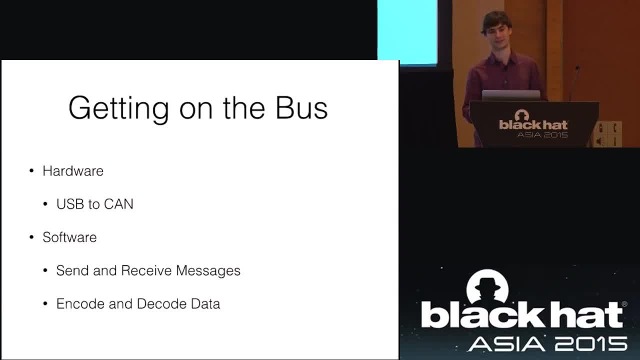 really uses anymore, And you'll also need a bit of software That just can make this easier for you to send and receive messages. Also, the software can often encode data into these formats. I mentioned CAN databases that define where all the bits are. 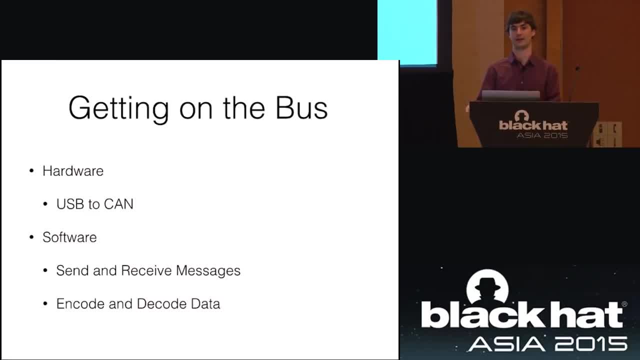 and what they mean. There's tools that will take live CAN data and decode it into real world values. So you just look at engine RPM temperature. all this stuff just shows up. So with a little bit of hardware, a little bit of 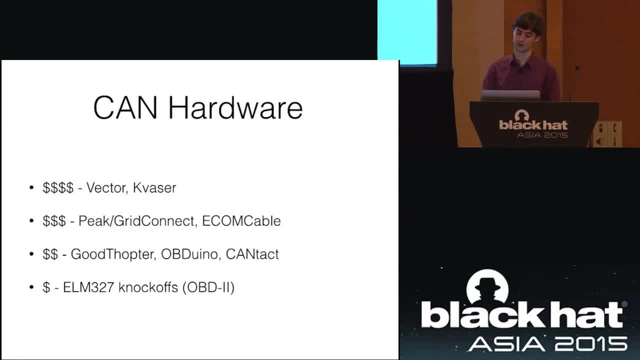 software you can hop on a CAN bus. So we'll start with the hardware part. Unfortunately, a lot of this is kind of expensive. Vector is like the holy grail of CAN tools. They're like the really expensive company that OEMs. 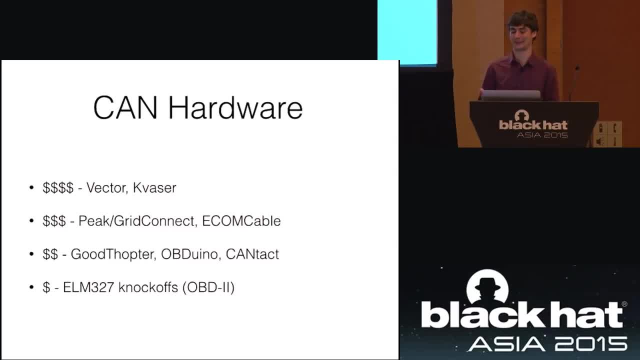 use and not many other people, Because the way I explain them is it's so expensive they don't list the price on their website. You have to call them and ask. Kvasr is another pretty expensive tool. They're also a pain to work with. 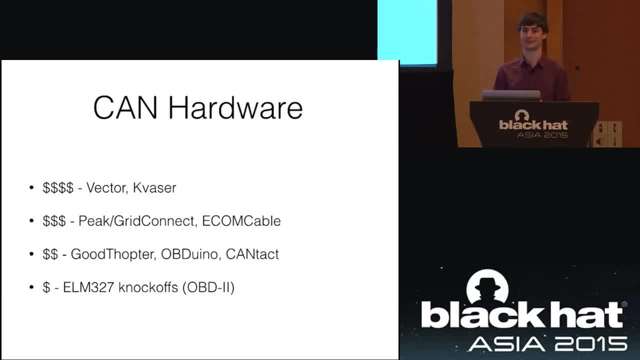 Moving down in the price list, you got peak, slash, grid connect- Same thing with a different sticker on it. That's $250, $300.. This one's not bad. It's got some support for socket CAN, which we'll talk about later. 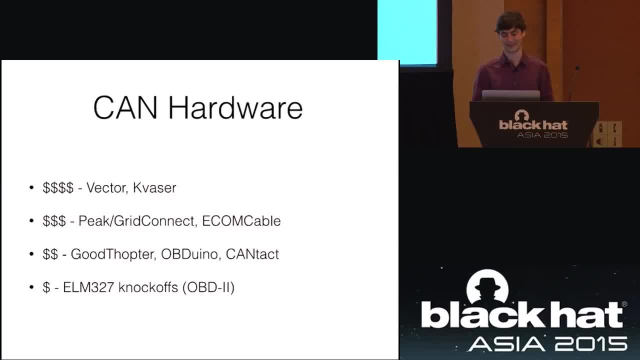 But it's not the best tool I've seen out there. It's got some weird issues with VMs. in particular, There's the ECOM cable, which I haven't used, but was used by Charlie Miller and Chris Valsek in their research. 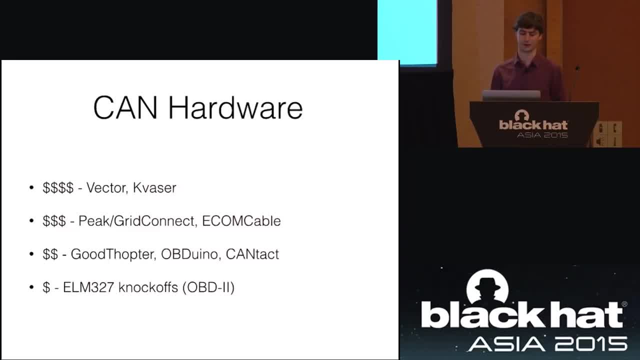 And it's $150,, I think, for that tool and it just gives you an interface with you take some DLL and you can write your own scripts for it. Moving down in price, you got the open source options, which include the Goodthopter by a guy named Andrew Ryder, which 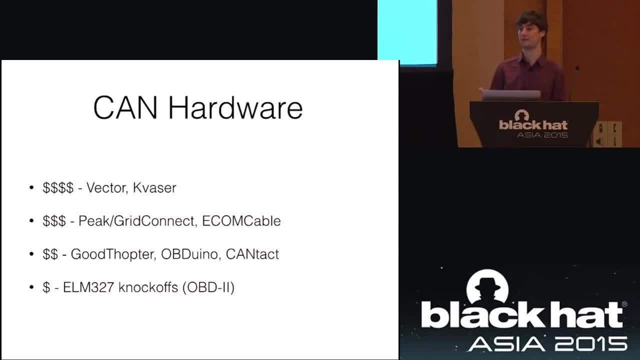 it's actually the Goodfet. If you've seen Travis Goodspeed's Goodfet, it's that for CAN. And yeah, it does CAN to USB for you. Only problem is you can't really buy them. You can get a board and solder it up yourself. 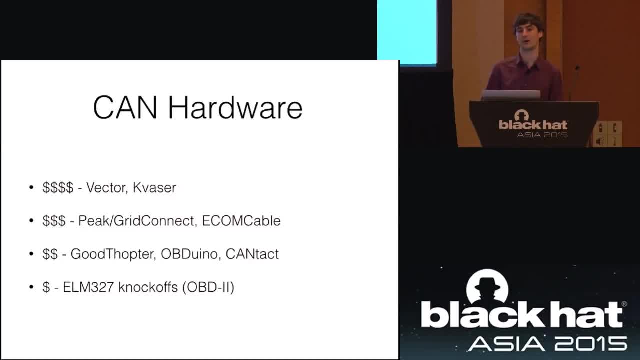 OBduino is sort of the same thing. It's an Arduino clone. that was a really, really good idea, I think originally meant to be like a DASH unit that you could read OBD messages, which we'll also talk about later- and 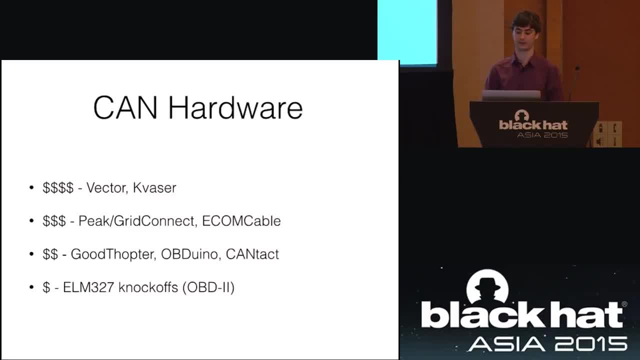 display them for you. Again, you can build one of those yourself. And then CANtact is a tool that I'm working on, which we'll talk about later. that looks like this And USB goes in one side, CAN comes out the other. 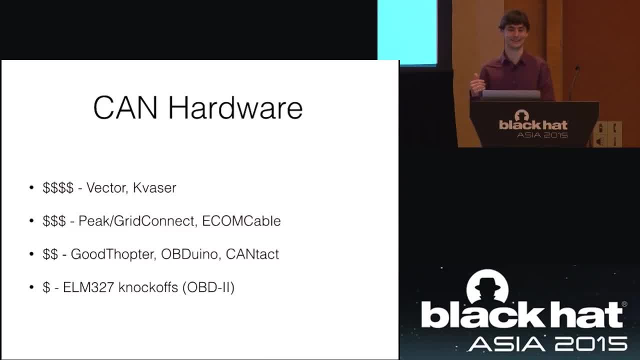 Last one are these Elm 327 knockoffs, which are kind of neat. These do a bunch of protocols that are for OBD2.. It's not always CAN OBD2, it's this diagnostic protocol that uses five different electrical signaling things. 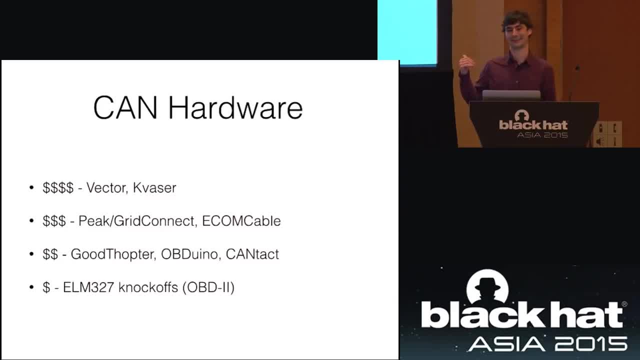 depending on the car, It'll do all of them And you can get these from Deal Extreme for $10, which is pretty fun. If you just want to play around with it, go to Deal Extreme and buy one. There's no reason not to. 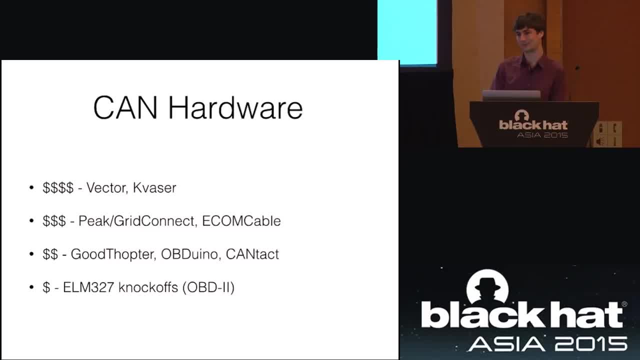 I recommend a USB one instead of a Bluetooth one, though, for all the reasons that we're discussing. On the software side, you have the proprietary tools, But really I don't care about those. They're expensive And we're focused on the free ones. 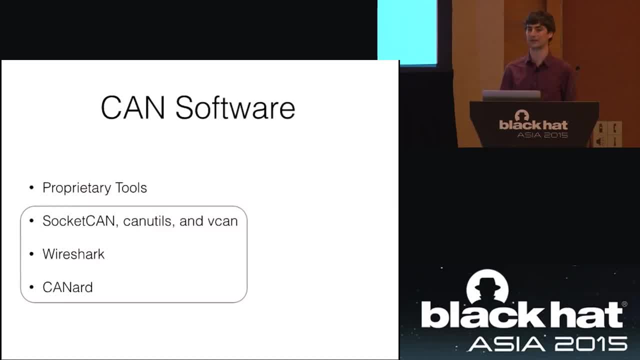 So SocketCAN, CANutils and vCAN- these are some things built into the Linux kernel. You've got Wireshark, which is something you've probably used for looking at IP networks, But we can use it for CAN too. 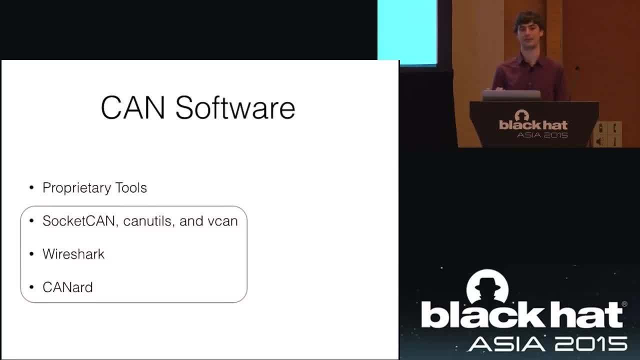 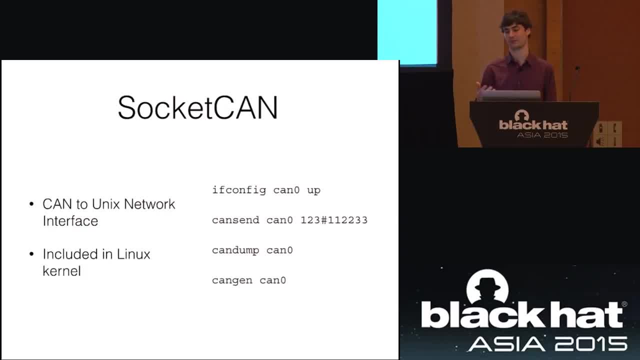 You can do a Unix network device like a typical ETH0, except it's CAN0.. And you can literally interface with it using ifconfig. And it's great, You can even do routes if you want. to. which sort of works. 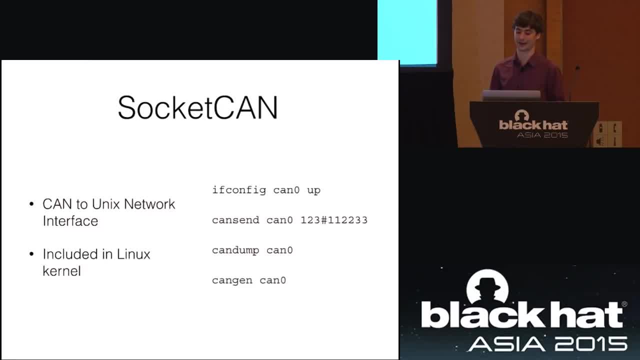 And once you get that working, you can use the CANutils package to use these tools like CANsend, CANdump and CANgen, which we'll take a look at. One nice thing is this is now included in the Unix kernel or in the Linux kernel. 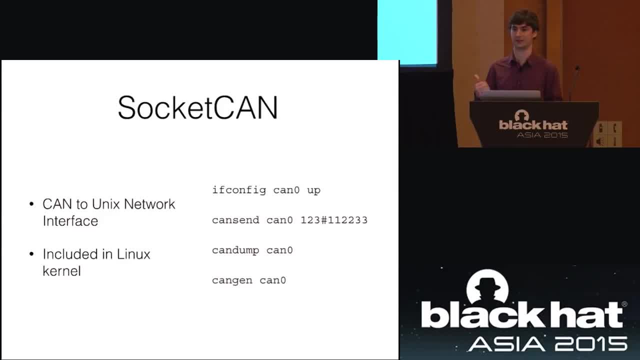 By default. if you install the latest Ubuntu, this is in there. you'll have to type, maybe modprobe something You don't even need, that actually It just works, And then you can apt-get all these tools, which makes it. 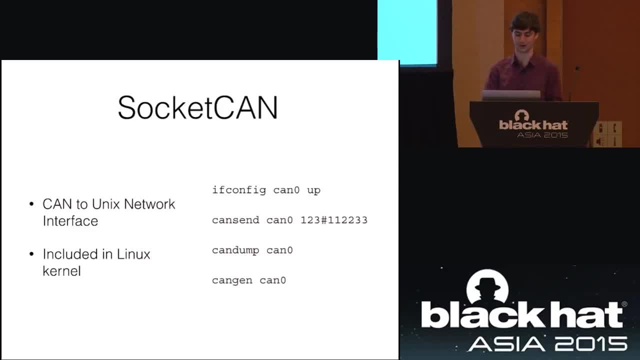 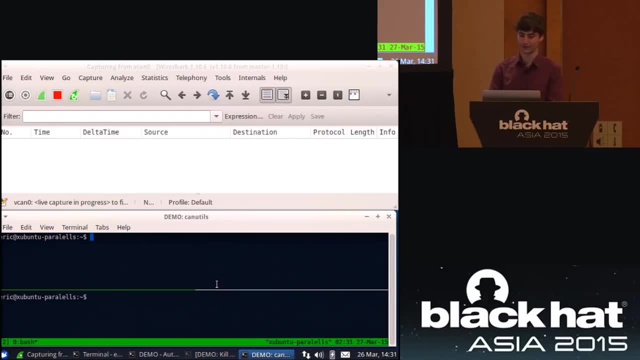 really easy to work with, rather than you don't have to build anything from scratch. It just works, And so I'm just going to show what that looks like just really quickly. These are simple tools, But I have Wireshark up at the top. 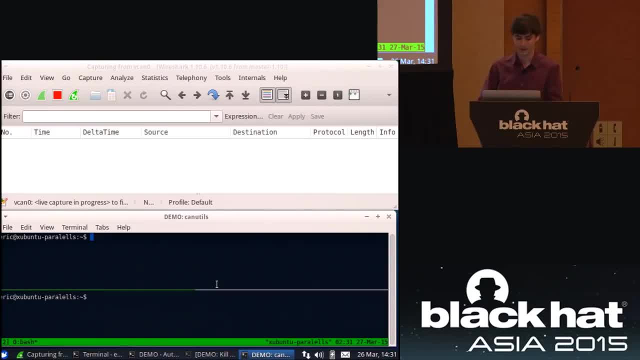 I'm sorry, the resolution's a little sketchy but hopefully legible. Wireshark's up the top which will show us what's going on, And I'm going to use the vCAN module. So vCAN rather than sending real messages and receiving. 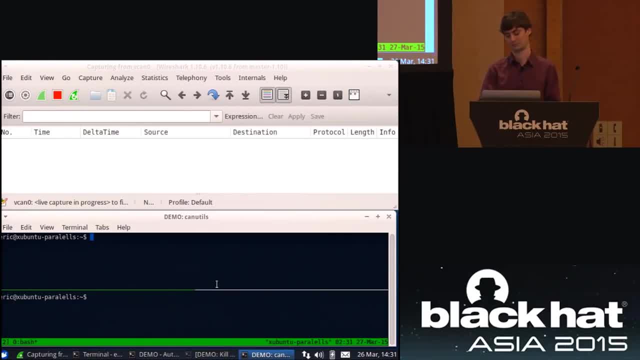 real messages just lets you do it all in memory And it's just a local virtual CAN device. So if I just do a CANgen vCAN0, we'll get some traffic And Wireshark will nicely present that And you can take a look at it. 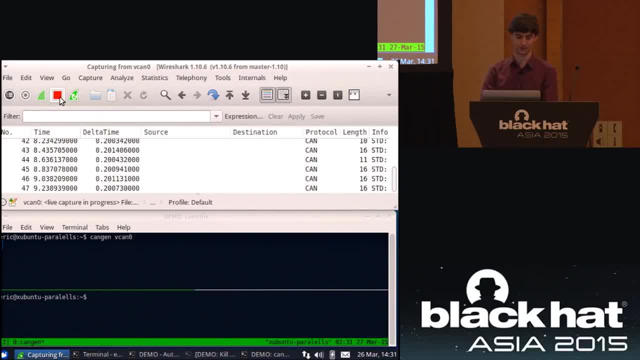 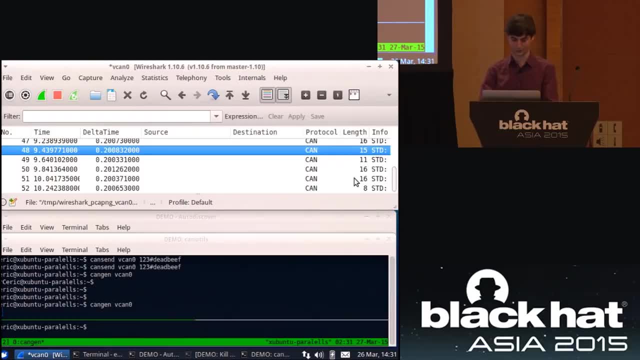 Sadly we can't see all the way across, But you will see the typical what you'd expect to on Wireshark data length. The ID is over there. Well, let me get that far over. But yeah, it's just an easy way of dumping that data. 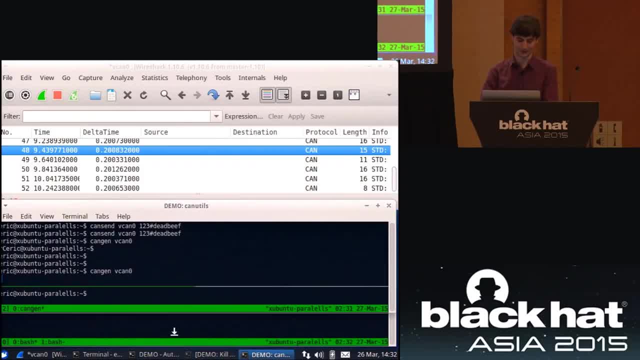 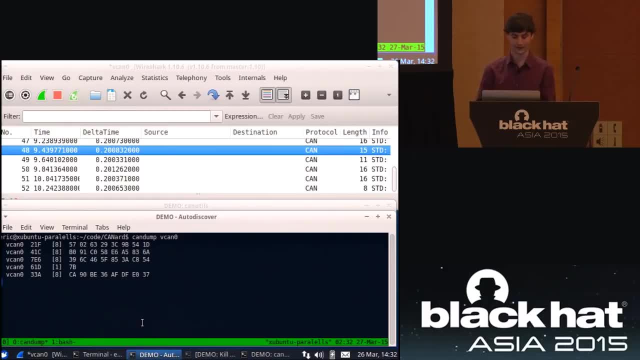 If you want to do it in an even simpler way, you can run. I've resized my window. We can run canDump vCAN0.. And this is just going to dump out all the messages. If you plug a device into a car, though, and do this, you. 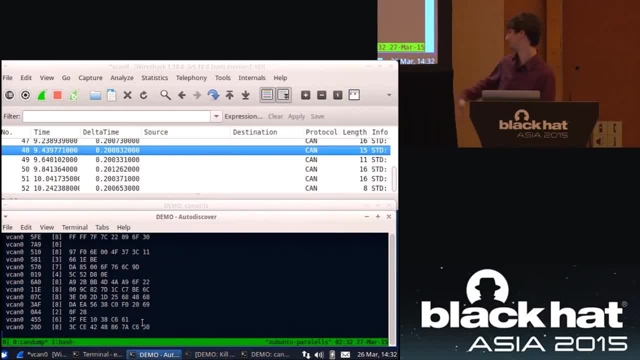 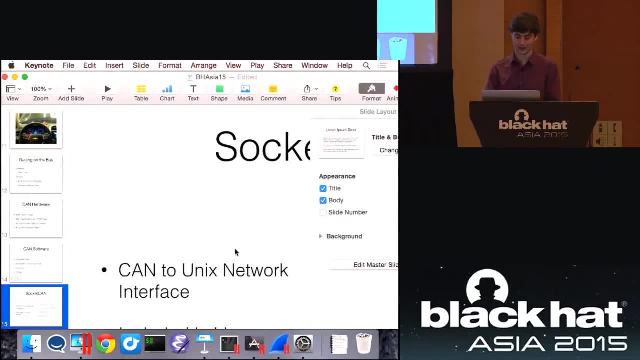 will get a very, very fast rate of data, with a whole bunch of real live car data flying by, And Wireshark is just a great way to be able to filter that stuff out. So on the topic of Wireshark, it not only lets you see, 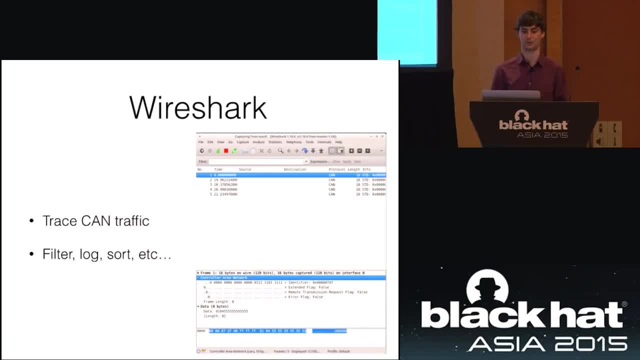 what's going on, but it also lets you do everything you'd expect to do with a normal IP network. You can actually filter based on ID, You can filter based on data lengths, You can put in columns for delta times to see time differences. 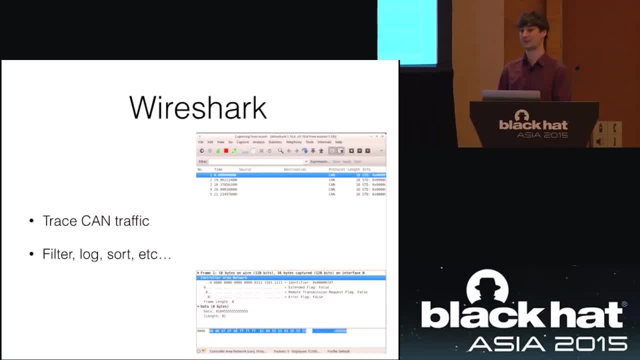 You can put in everything that you'd expect, And you can also save packet captures, replay packet captures, So it's a really great tool. It actually is more powerful than most of the proprietary CAN tools for doing the same thing, which is great because 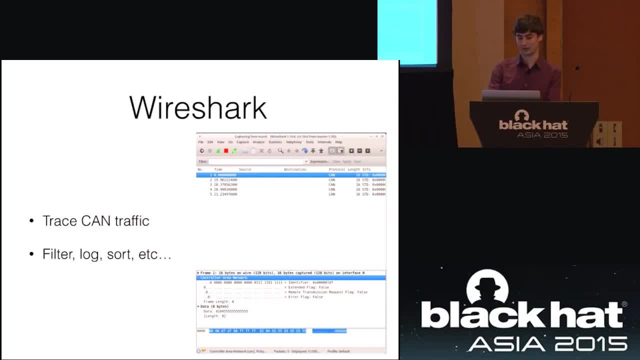 it's free And I've been using this actually for work a lot, because you can write custom CAN scripts for interfacing with whatever system and then just fire up Wireshark in the corner and it will just tell you what's going on in the bus. 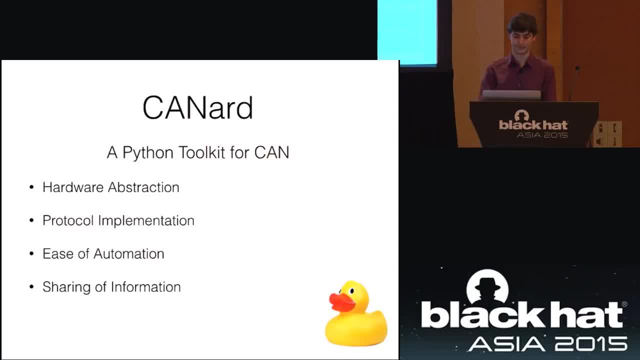 at all times, which is quite handy. Then we get into some custom steps. So I started playing around with this and realized that there's a lot of little scripts out there, but there was nothing I could really build off of. So I decided to build my own little Python toolkit for CAN. 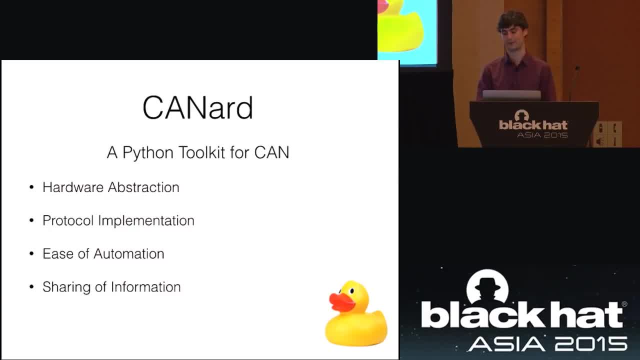 called Canard, which is French for duck Vector, stole all of the CAN puns from me. They have canoe, canalizer, canopy, they also have the candela Can-de-la, So they stole all those. so I was stuck with French. 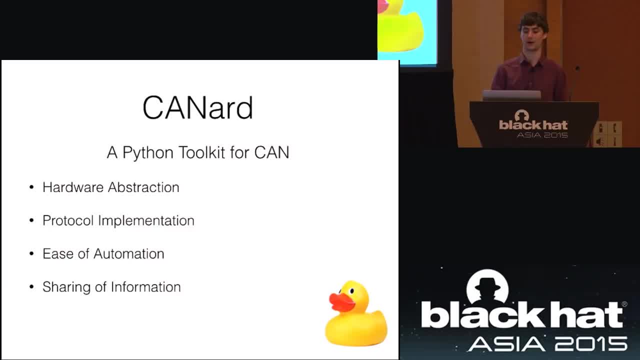 But the idea of this software is to provide some hardware abstraction to implement the protocols that are really common on these CAN buses, to ease automating looking at CAN buses and sending and receiving messages and also just to make it easier to share these things. 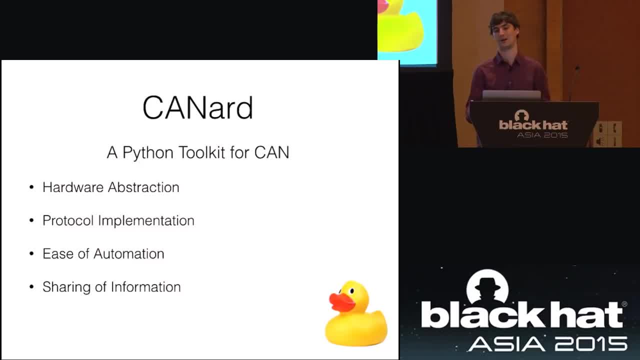 If the hardware is abstracted and you have any supported tool, now I can give you a script and you can just run it and it works, rather than: oh well, you know, I've run it and it's working. It's working. 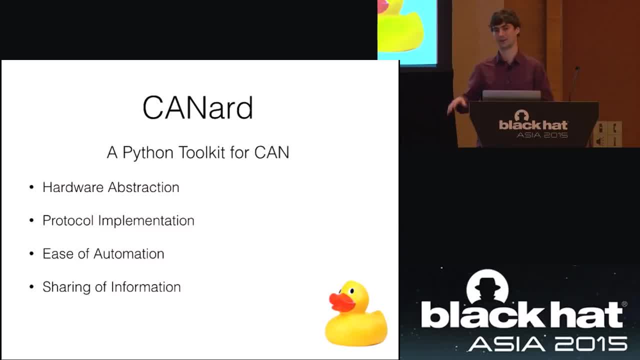 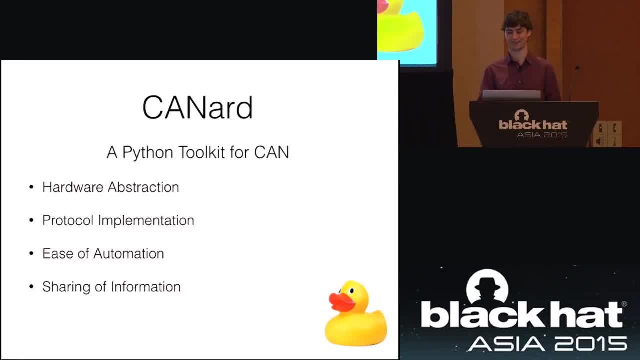 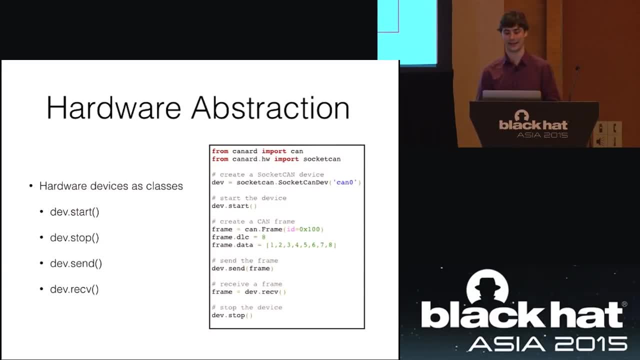 the people who actually make those tools means that you can make it compatible with all the tools, which is nice. So what do I mean by hardware abstraction? Well, really simply, a hardware device is a Python class that has to implement four methods. 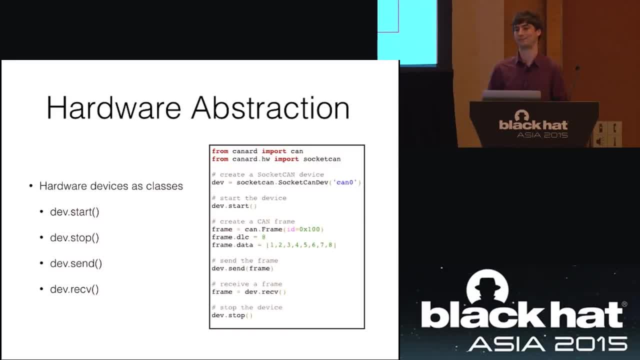 Start, stop, send and receive. It can implement more to do things like set bit rate, things like that, but really this is all a CAN device actually needs to do in the most basic form. So a really simple code example if you're wondering. 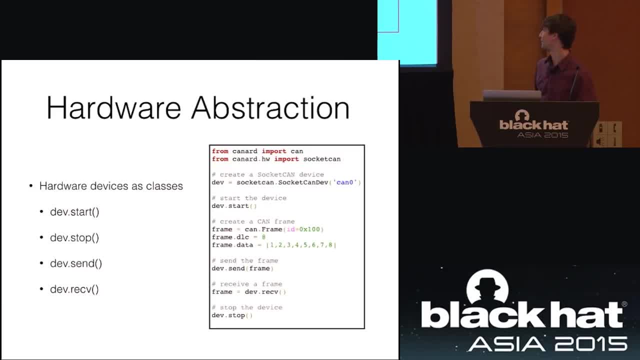 how you actually do this is: we import some stuff. We're going to create a socket CAN device. So this is going to bind to the CAN0 device as a socket. We'll start that device with devstart, Then we'll make ourselves a CAN frame. 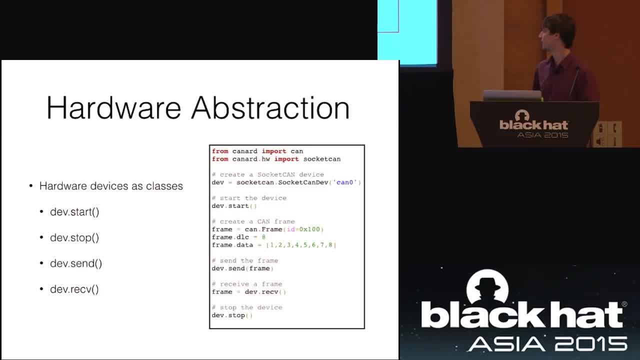 So that is a frame with ID 0.. That's the identifier. The data length code DLC is 8, saying that it's 8.0.. It's 8 bytes long And the data is 1 through 8.. 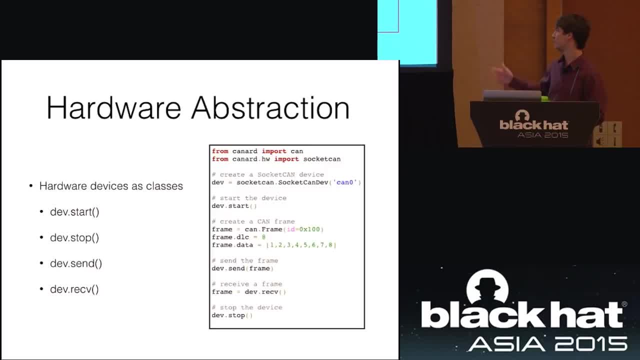 It's not a terribly useful frame, but it's a frame And then we can just do devicesend or devsend frame and it will go out on the bus To receive a frame. we just do devreceive and we get a frame back. 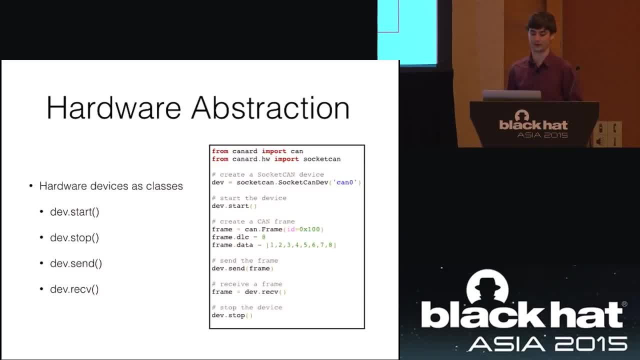 And then finally, when we're done, we can stop the device and free it up for other stuff to use. So really, with those four methods implemented, you can now write more complex protocol stuff and have it work. You can work across different devices. 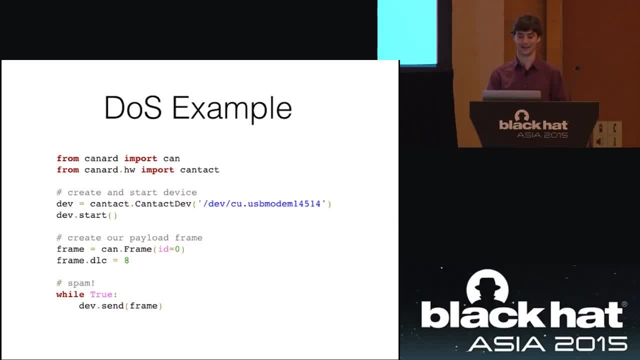 which is what we'll get into next. But first I talked about this denial of service thing And I really like it whenever an example that does something, especially something bad, fits on one slide. It's great when the code does that. 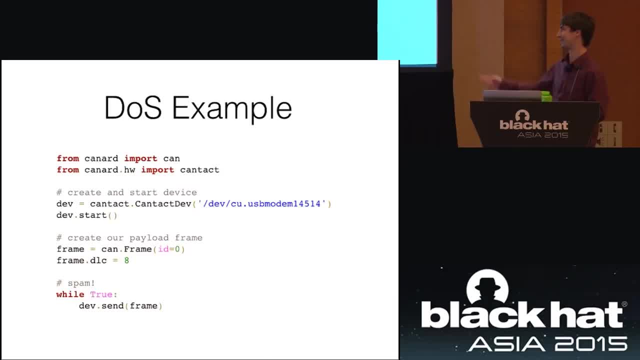 And I mean this is pretty much the same as the last example. Only difference is ID is 0. We set the length to 8, just because, while we're spamming the bus with 0s, we might as well spam it with as many 0s as possible. 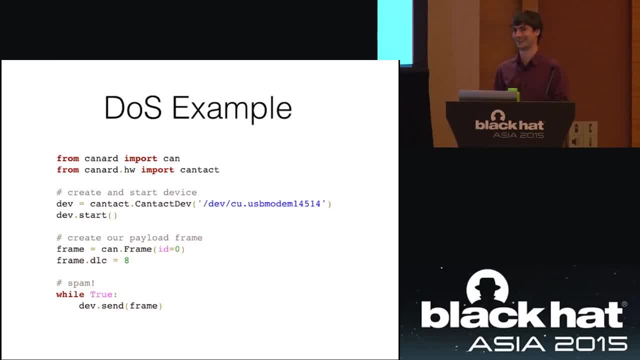 So we just had to do that. We set it to 8.. We don't care what the data is, As long as the ID is 0, it's just going to shoot out 8 bytes of data. And then you know, wild truesend. 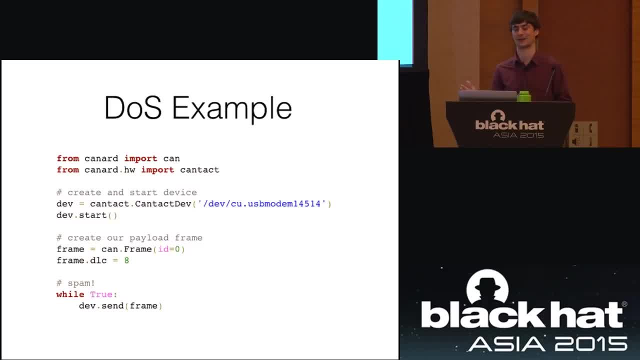 This will send many, many frames a second. It'll totally lock up the bus. You will latch fault codes on every controller because it will say I haven't communicated with the rest of the ECUs, the rest of the control modules in the car, in the last, however many seconds. 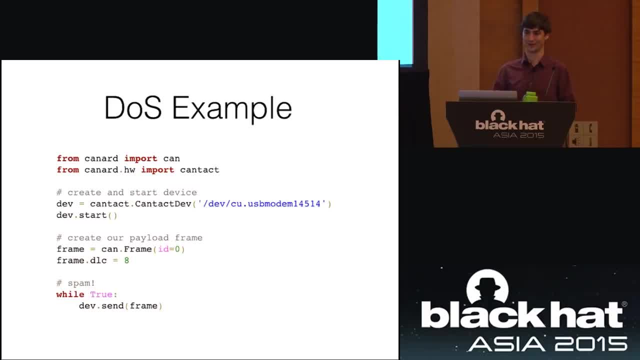 That's considered a hard fault, So you'll have to clear all those codes. It's really a bit of a pain, But it does work. In some vehicles it'll actually just totally disable things like it'll turn off the car, essentially. 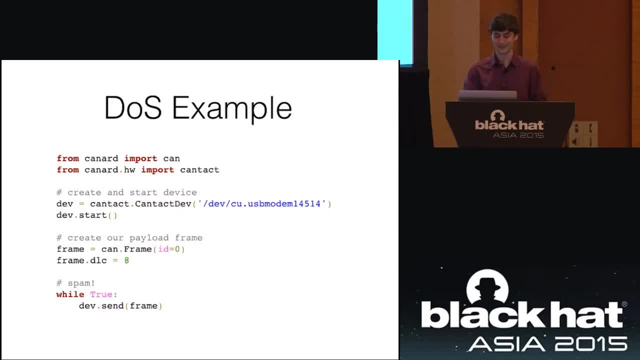 All depends on the car you're on and what CAN bus you're on, But it can do some nasty things. So now that we've talked a bit about CAN and just the simple injecting messages and sending messages at high speeds, we're going to get into the fun bits that the 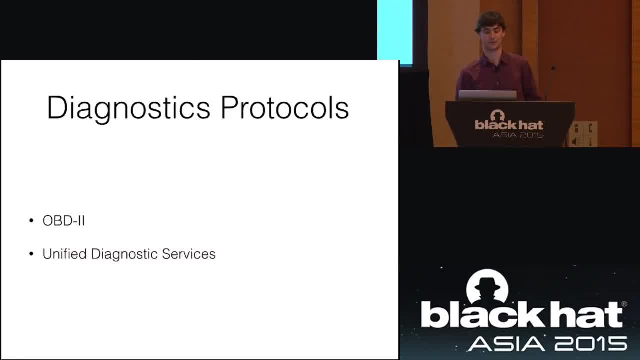 manufacturers don't tell you about which is the diagnostics protocol. So there's the diagnostics protocol. There's really two main diagnostics protocols. One is OBD2.. And one is Unified Diagnostic Services. Conveniently, OBD2 is a subset of UDS, Unified Diagnostic. 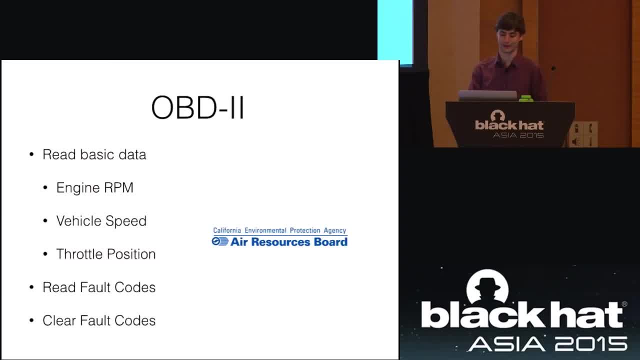 Services. So we can start with OBD and build And OBD. it's actually courtesy of the California Air Resources Board. They decided that every car sold in California had to have this back in 1991, because they wanted to be able to do smog tests. 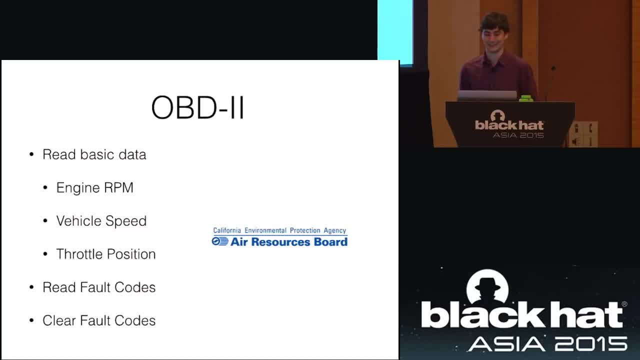 So they mandated it and now every car has it. It lets you read basic engine data, the vehicle RPM, throttle position, vehicle speed, math, pressure, so on and so forth. It's all read-only that stuff. It's interesting if you're trying to tune a car or fix a. 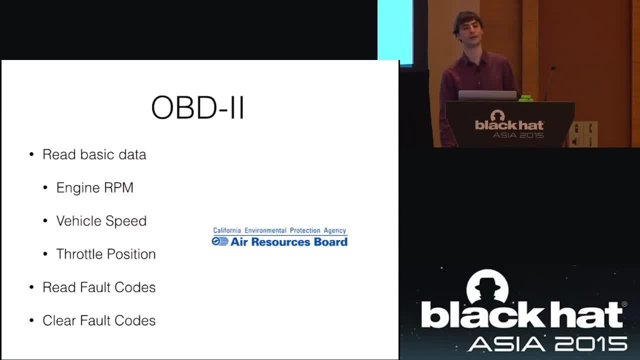 car and see what's going on. That's about it. You can also read the fault codes. This is actually a really great way to save money. If you read your fault code and see that's a dead mass airflow sensor, You can just replace your mass airflow sensor. 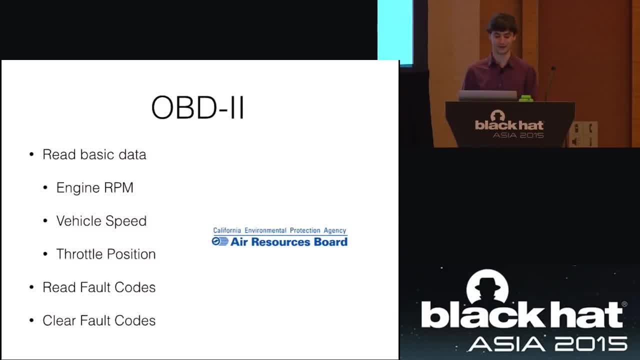 and then your car usually works again And you can save yourself a trip to the dealer. But you can also clear the fault codes. So when that little lamp comes on with the check engine, all that means is that there is some fault code somewhere. 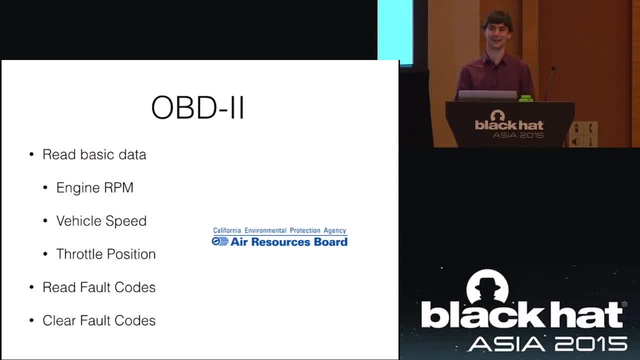 And this lets you not only read them but clear it, And that's really all it does. Not terribly exciting, but somewhat useful for just looking at vehicles and getting some basic information. Another important thing about OBD is that they standardized this connector. 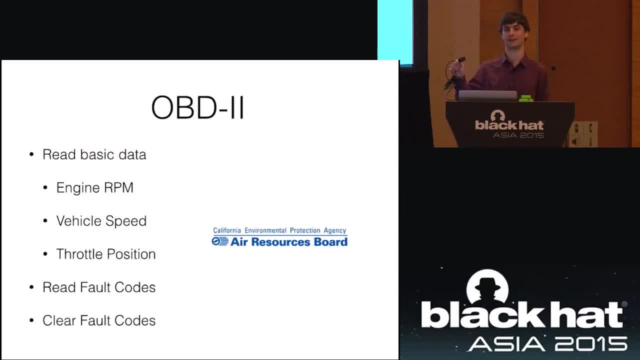 It looks like that Any car you get in is going to have the mating side of this connector under the dash, typically by your knee somewhere if you're driving, And that will give you access to a few things- at least one CAN bus in modern vehicles. 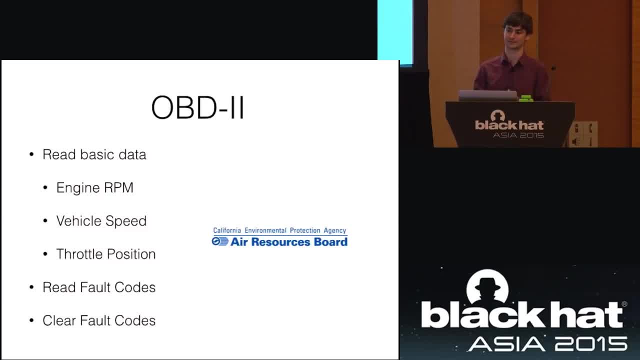 Anything past 2008,. like I said, is going to be CAN for diagnostics, so it's going to have at least one CAN bus. What's kind of important about those connectors, though, is they only specify some of the pins. The other pins, manufacturers just kind of do their own thing. 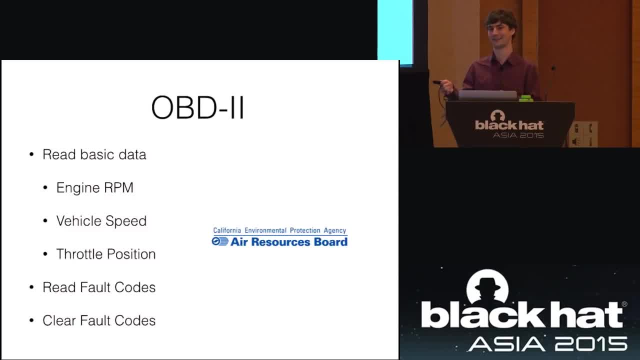 Back to the Volt. actually it has two ports, one on each side of the car, But they conveniently break out every single CAN bus to one of those ports So you can just hop on to any of them really easily. Really convenient when you want to do data logging or look. 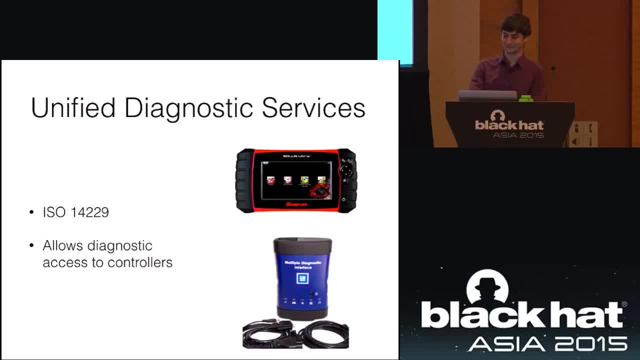 in more detail at those. But OBD, it's kind of neat, but it's not the big picture. Unifiedcom- That's the big picture. Unified Diagnostic Services is. It's this ISO standard 14229,. if you want to Google it. 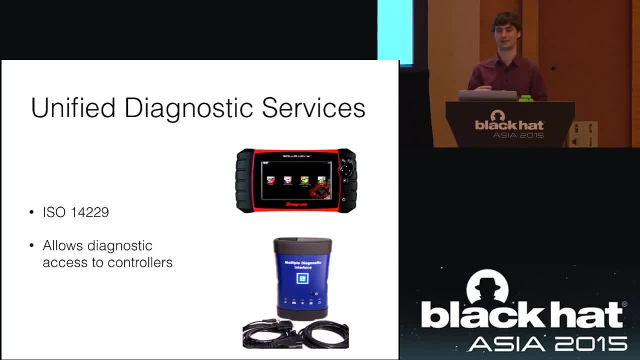 And it defines a diagnostic system that is used by every automotive manufacturer. The reason is because when you take your car to a mechanic, they're going to use a tool like that thing up top- the Snap-on Scan Tool- to take a look at it. 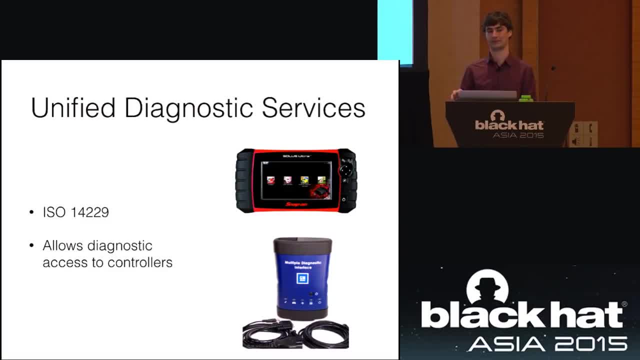 Now they don't just get OBD, They get another set of messages that's manufacturer-specific, But that manufacturer has to provide them a database, And this ISO standard basically says: here's how you're going to communicate for diagnostics And here's how you're going to provide the database. 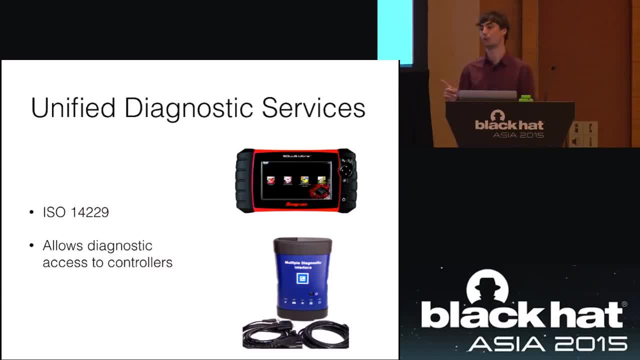 to the people who make these tools. That way, Snap-on can build one tool that can do Mercedes, BMW, GM, all those- because it just has to speak one protocol. It's also really handy when you want to reverse engineer these. 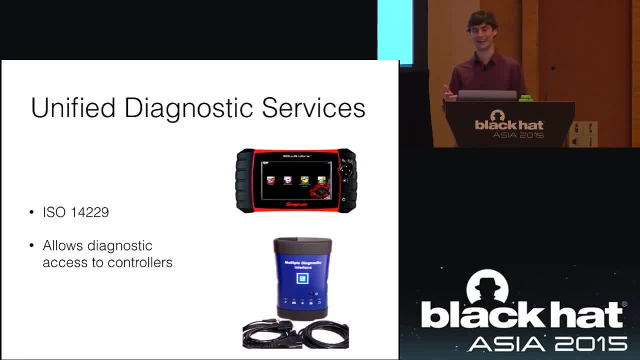 because there's an ISO standard that tells you what the protocol looks like And you can just implement it yourself. So yeah, usually you would have to buy a rather expensive tool like the SOS Ultra from Snap-on or the MDI from GM that can do this. 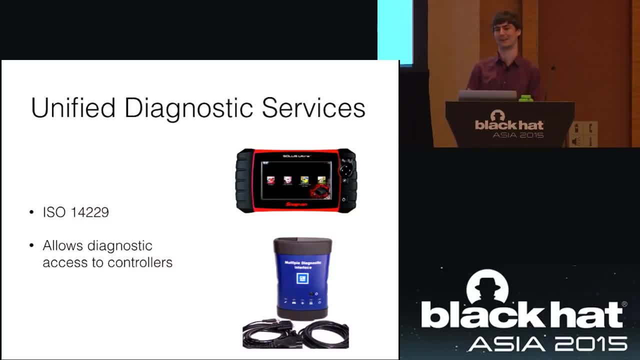 Then you have to pay a yearly subscription in order to get those messages, And that's just a subset. That's just the messages that are considered for mechanics. There's a whole bunch of other messages there for the OEM that are way more interesting. 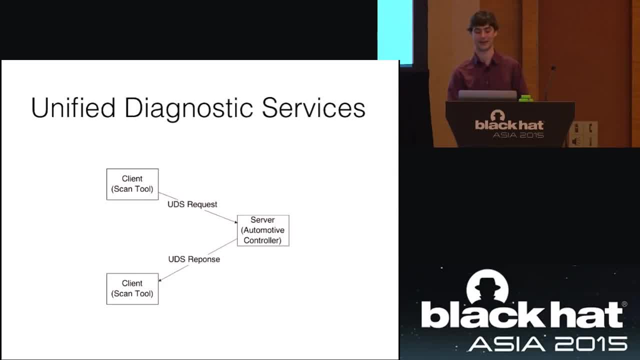 But how does this work, this ISO protocol that everybody uses? It's super simple. You have a client like that tool, You plug it in. It sends a UDS request and then a server. This is their ISO terminology. The server is that controller, maybe an engine controller. 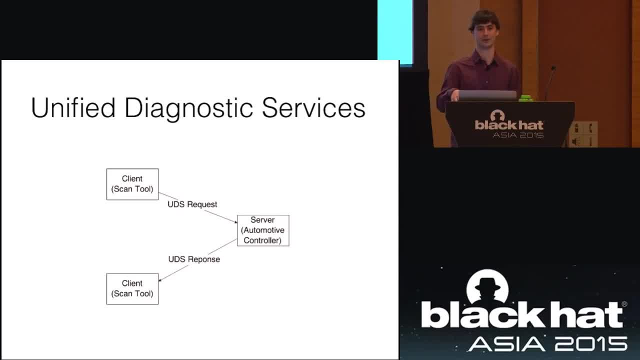 maybe a body controller, maybe a door handle controller, if you have a Tesla Model S, And that server will send back a response. That's it, Really simple. All you have to do is figure out how to pack the data and you can send requests and response all day. 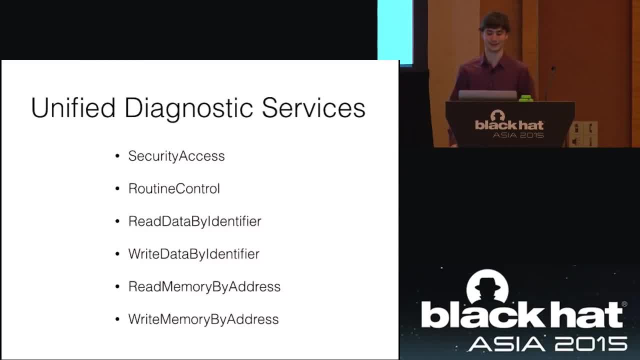 And what kind of services are we talking about? They're unified and diagnostic services, But this is a short list. There's actually something like 30 of them. These are some of the cooler ones, I think. So security access, we'll talk about a bit. 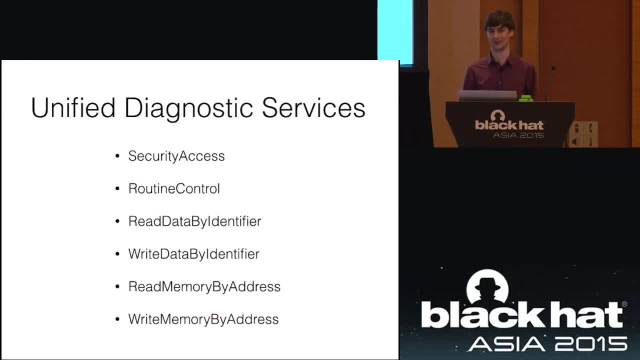 But this lets them provide a basic level of security. It's really basic and we'll show that it's broken. It's been shown to be broken a few times. The routine control is a way that you can just run arbitrary routines on the controller. 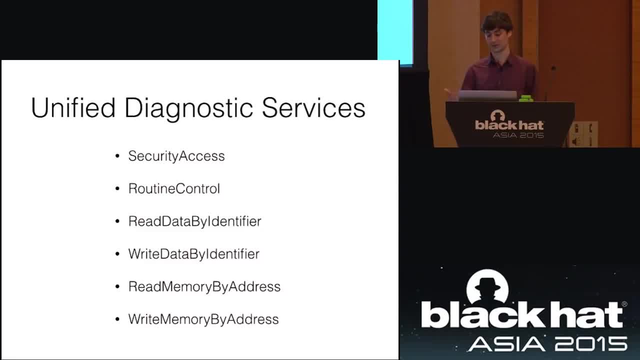 The idea is, if you're servicing a car and you want to find out why a window isn't going down, well, now you can just actuate the window from your scan tool. You don't have to just push the button. So now you can isolate things. 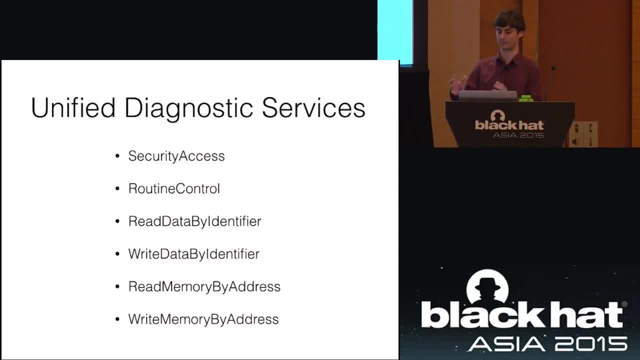 You can say: oh well, the window goes down when I ask it to with my scan tool, but the button doesn't work, so the button's probably broken. A lot of things like that, where you can just do diagnostics step by step and isolate little pieces. 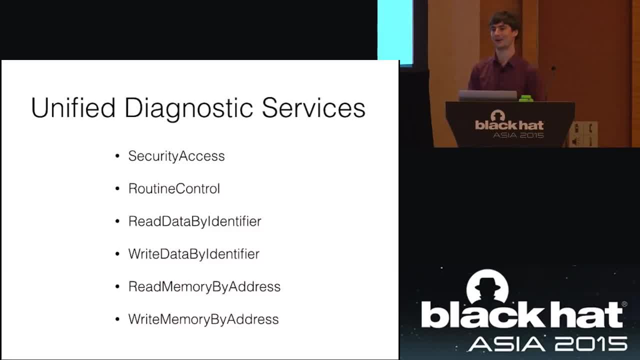 Read and write data by identifier. This sounds pretty arbitrary, and it is because these identifiers identify everything from the VIN number of your car to its lookup values for the engine, so that it can do different emission standard stuff to everything you could imagine is one of these values. 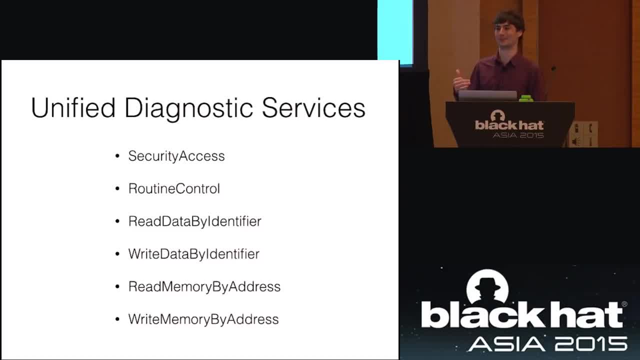 And you can read them and sometimes you can write them, which is kind of cool, especially with things like VIN numbers and engine Control values and things like that. And then there's also the memory access which is implemented on some controllers, which literally 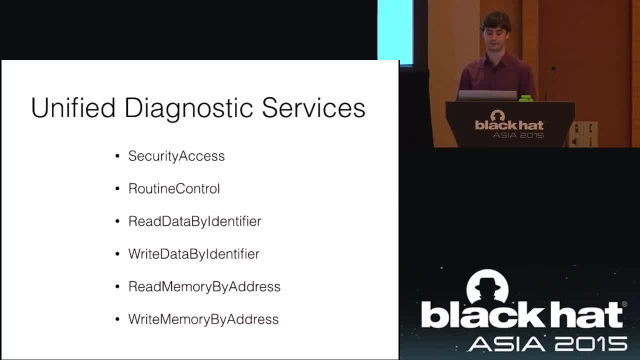 just provides you arbitrary access to memory. This is in most cars I've seen, somewhat locked down, But with so many cars out there and often these implementations being done by one company that hands it off to another company that hands it off to another. 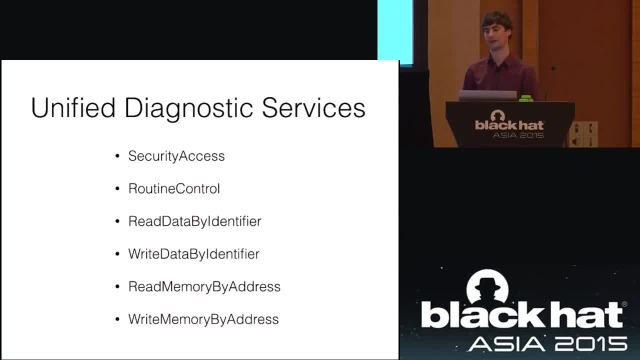 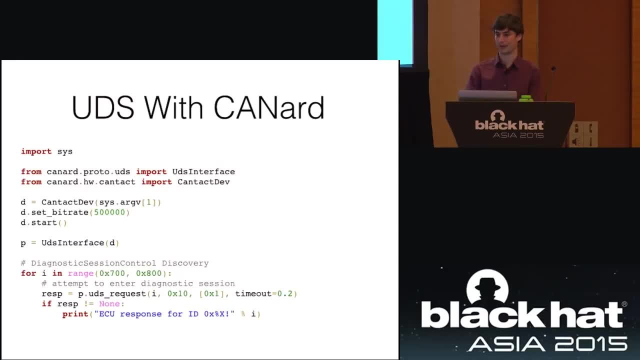 company that finally puts it in the car. there's definitely going to be edge cases with all this stuff when you start scanning for it. Talking about scanning for it, that's one of the things that was really lacking I found with most of the stuff out there was it's an ISO standard. 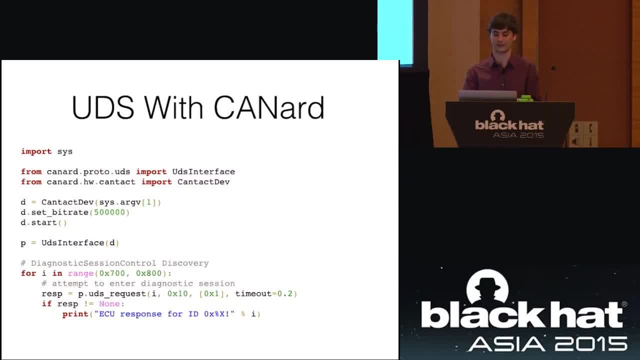 It should be really simple. There should be software tools out there to send and receive messages. There really wasn't anything out there where you could just say: OK, I want to do UDS and I'm going to tell you the service and the payload. 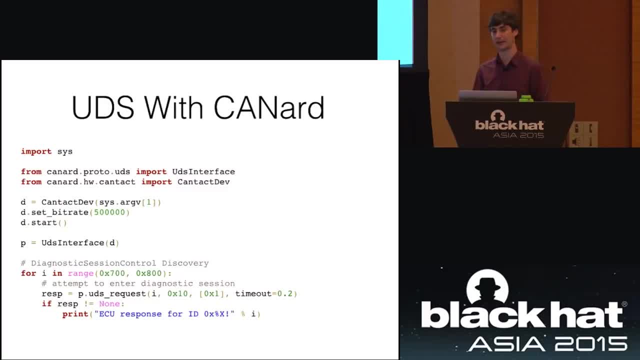 and do it for me. So this Kennard tool, I've built that into. So what this does is it starts up, imports some stuff and then it's going to create a device. I used the CanTac device, just to be different with this one. 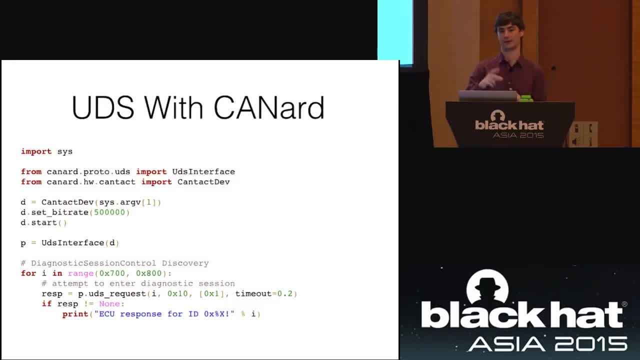 This is a direct access to this board rather than going through socket can. The reason for that is you can sometimes have special features that aren't supported by socket can, things like listen-only mode and doing hardware level filtering by identifier, stuff like that. 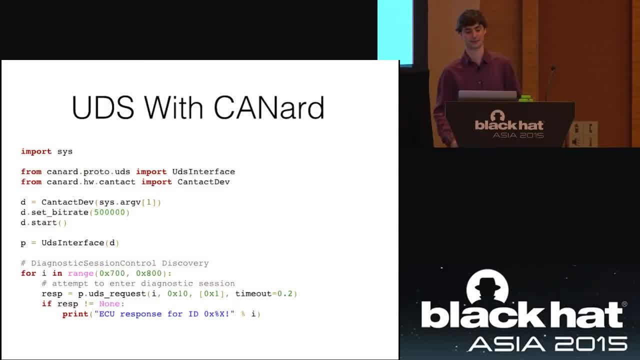 So Socket can doesn't support it, So sometimes you might want direct access. Then you can set the bit rate of most diagnostic ports. Actually all of them are 500 kbps. So you set the bit rate and you start the device. 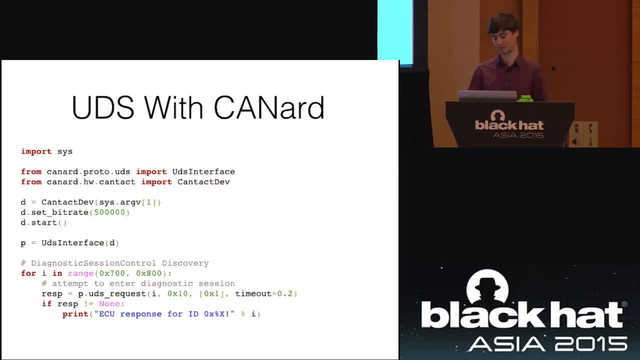 Then you just assign a interface, You just set up an interface And it actually takes over that device at that point. And then this gets really simple, because we can just send UDS requests and we'll get back UDS responses. So 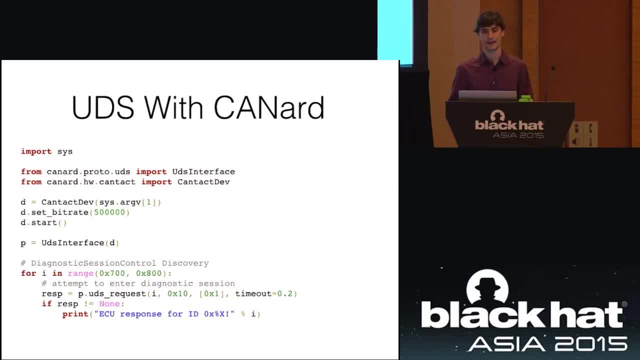 What I wanted to do with this example was I was plugged into a vehicle. It was actually a Honda. It was my roommate's- or is my roommate's- car, So I have to thank him for letting me plug into his car and mess around with it. 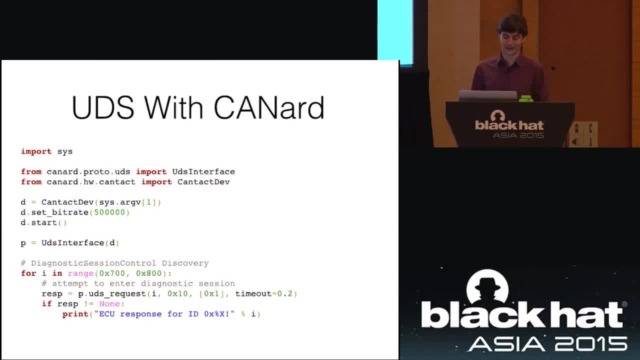 I did kill his 12-volt battery while I was doing it, so I feel sort of bad, But I wanted to play around with a Honda, because I'd never played around with a Honda And one thing is I don't know where to send my messages to. 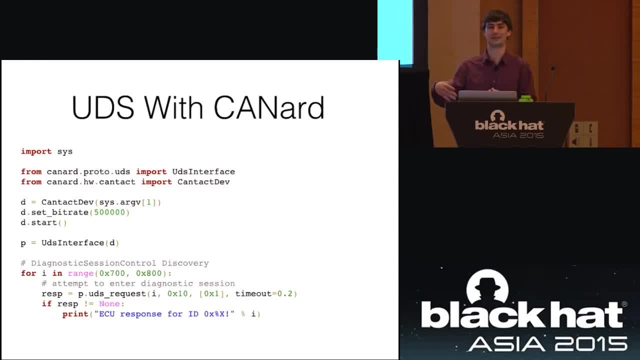 Where are the? you know what? where do I send my uh diagnostic requests to? I have no idea what's what a Honda's like, So I figured I'd scan and try to get a session diagnostic session from every ID on the bus. 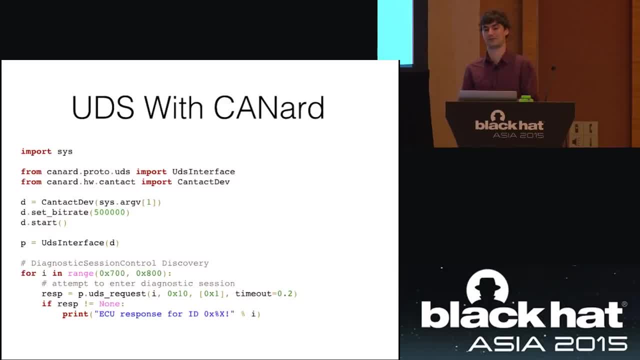 And once I get a response, a positive response, saying yes, you have started a diagnostic session, we're good, right, I found a controller And on Honda, it was really simple. I ran this and it goes. you see a response for ID 0x70.. 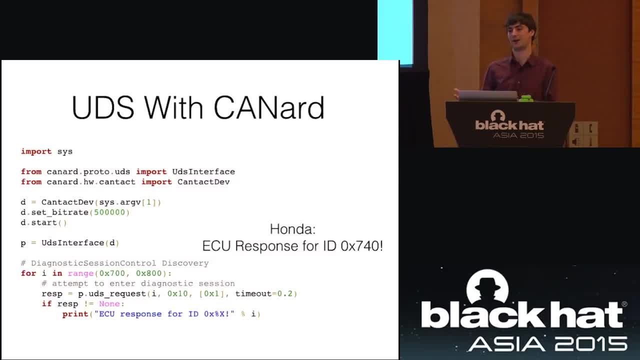 So what this is doing is it's going from 700 to 800.. I just know, having worked on these, that typically diagnostic messages are very high on the uh ID list of IDs, Reason being that whole priority thing: low messages get a higher priority. 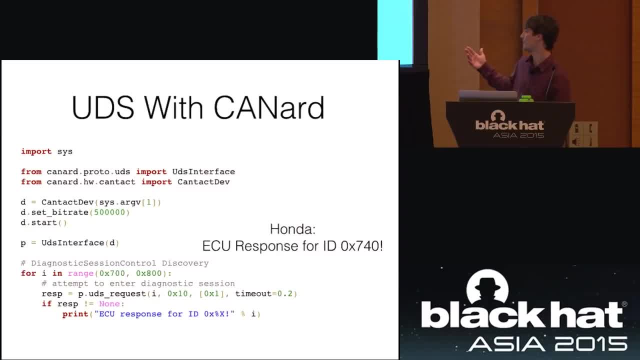 So they don't want diagnostics to be high priority, Then we're going to try to get a diagnostic session. So UDS request I is just the ID we're gonna send it on. Then we got the service identifier. 10 is the service identifier for a diagnostic session. 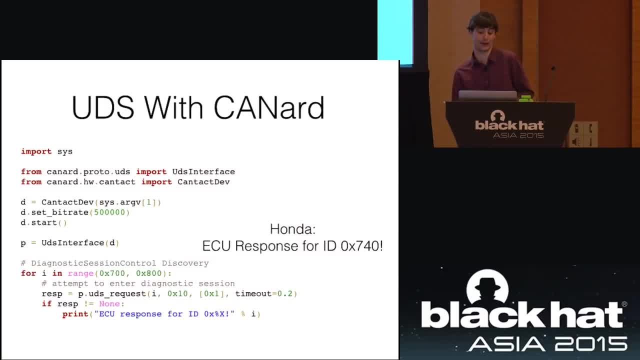 The payload is really simple for this. It's just what session would you like? I would like just the standard. OX1 is the default And the timeout is 0.2 seconds. That's actually a long time for this, but just to give the controller enough time to respond. 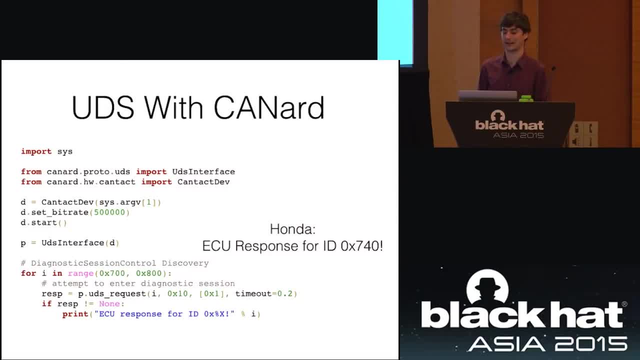 And then we just loop through it and send all these and wait for something to come back. And that's what I got from the Honda Some vehicles. I know GM puts way more on that bus, So you'd expect to get a lot more responses back. 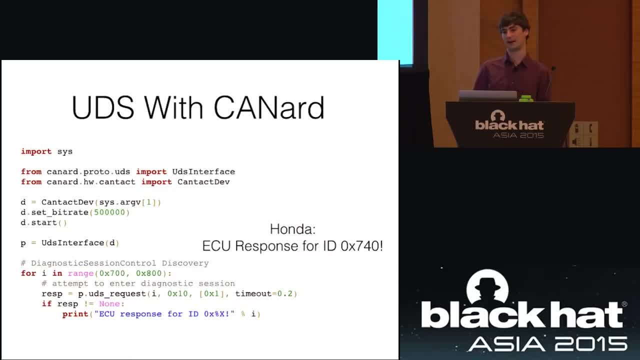 Same with. I believe Ford vehicles do the same thing. It really depends on the manufacturer. What some people have done is that OBD2 port. they've kind of air- not air- gapped it, but they put a controller that's immediately after it. 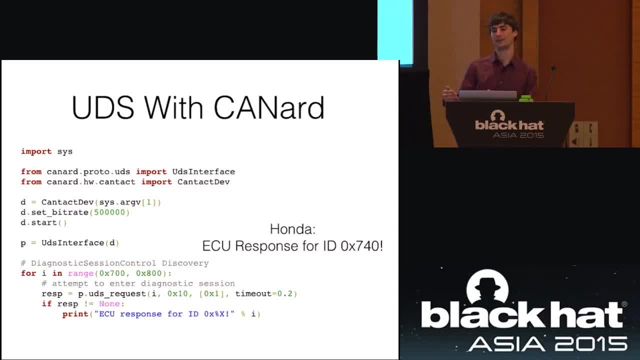 and made it so you can only talk to that controller. The reason is mostly because when people start putting weird devices on their CAN bus- things like these insurance dongles that Progressive will give you in the States, or Deja Day in Canada, or you know even little data loggers made by who knows. 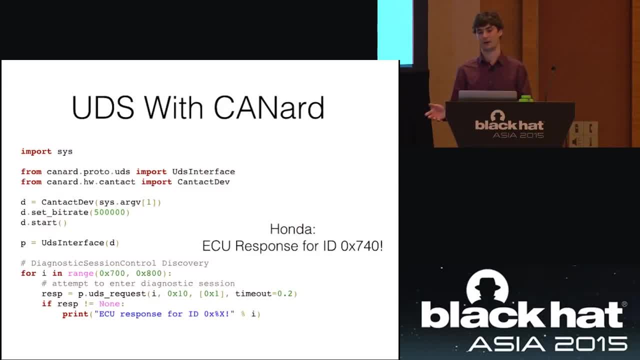 what company that might have some issues. The automotive companies don't want to be liable for those devices. obviously, If you're driving down the road and your car shuts down, they don't want to go. well, that was the fault of this little dongle that you plugged in. 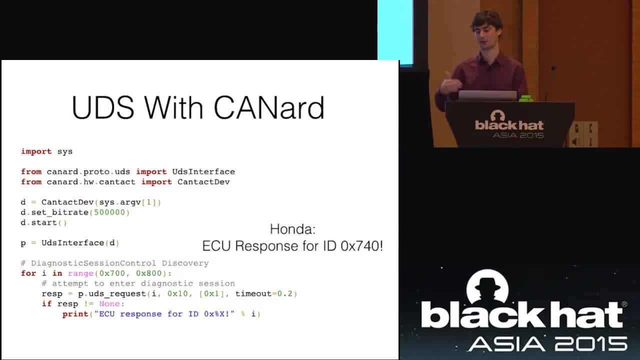 So what they've done is they've kind of created a bridge so you can't crash that the entire network, just by, you know, messing around with that first one. So in this case I only saw the one controller, but in a lot of cases you will see messages. 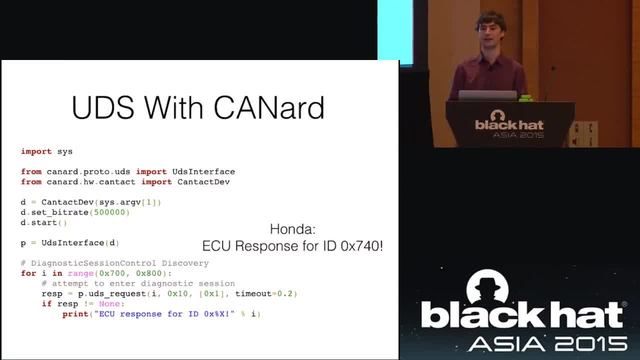 get gatewayed through that controller. So if you read an identifier, it might actually be from a different controller in the car and it's just working its way through and working its way back. So 740 is probably just a generic, you know access. 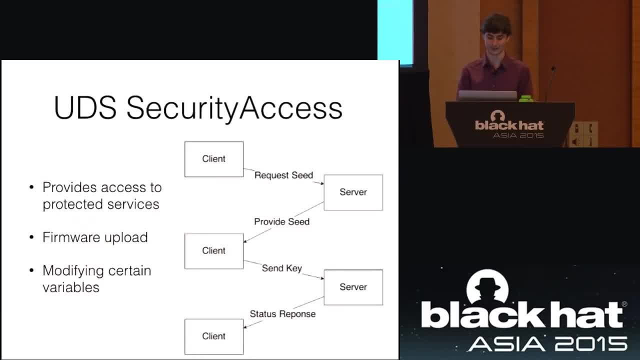 and you can request stuff from different controllers on it. Security access gets a special mention just because it's entertaining. Whenever they set this all up, they went well. OK, if we're going to provide access to read and write everything. 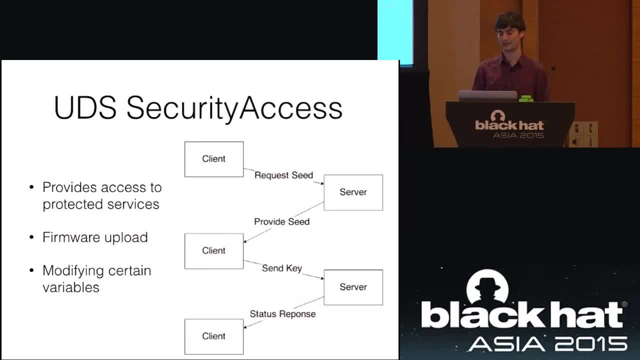 well, we should probably secure it, And so they set up this in the ISO standard, this security access thing, And it doesn't look bad in and of itself. It looks kind of like a normal seed key exchange. right, You've got a request for a seed. 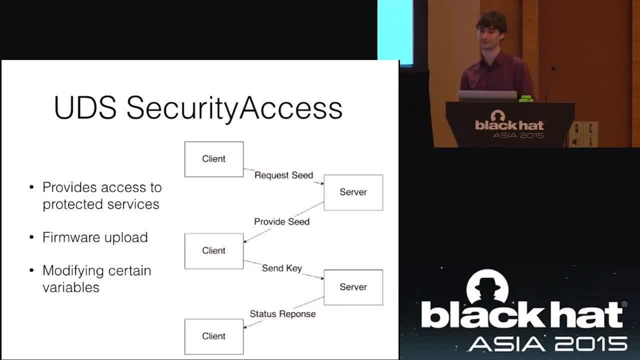 Then you get a seed back. From that, you generate your key. You send that to the server. It checks your key based on the seed, makes sure it matches. If it does, they say OK, positive response, You're good to go and I've unlocked myself. 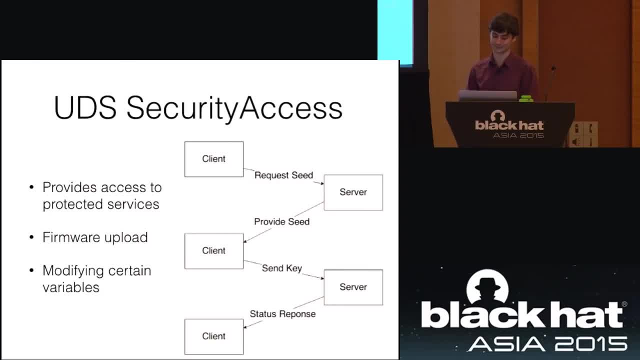 If it's wrong, it sends you back a negative response and you don't have access. Now, this protects some pretty interesting things. This unified diagnostic services is used to do end-of-line configuration of vehicles, So whenever your VIN number gets written into your car's, 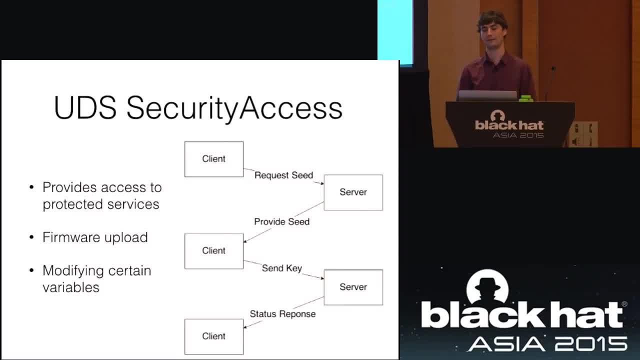 controllers. that happens over this protocol. In some cases, whenever firmware gets loaded onto controllers, that can happen over this protocol. There is a UDS service for upload and download data and it is used for writing firmware. So if you manage to get security access. 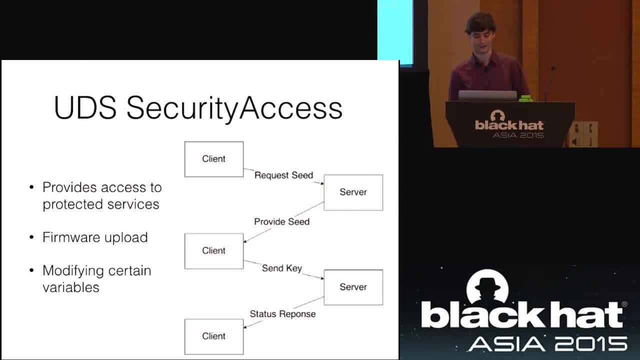 you can do some really bad things, But this protocol doesn't look terrible until you start breaking down some of the assumptions they've made. The first one is: the seed is fixed. Now, the reason that they give for this is that they didn't want to put the algorithm or some. 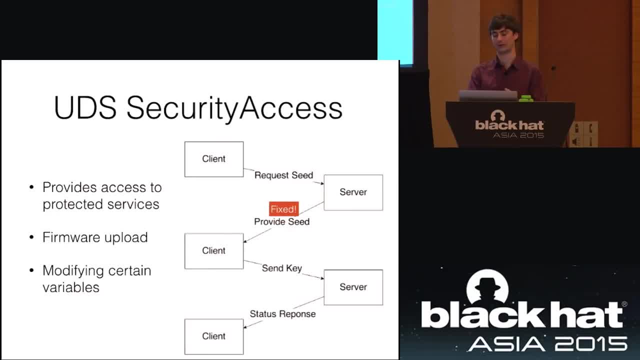 actual important key in every controller. So instead they just put one seed in every controller and it'll just send you the same seed every time. So, OK, that already means one thing, which is that the key is fixed, And that means this is 100% vulnerable to a replay attack. 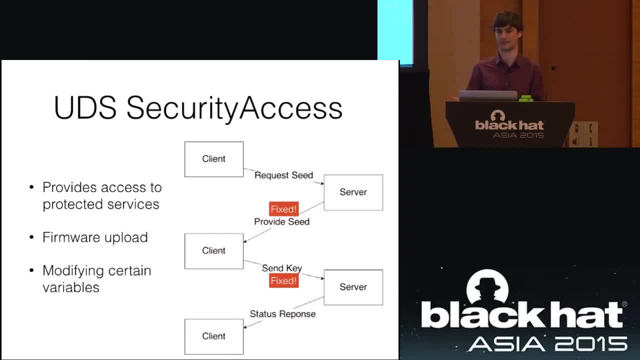 because it'll just send the same key back every time. You don't even need to look at the seed. You know it's the same thing. Still not so bad, because odds are, unless you're logging the bus while a firmware update happens. 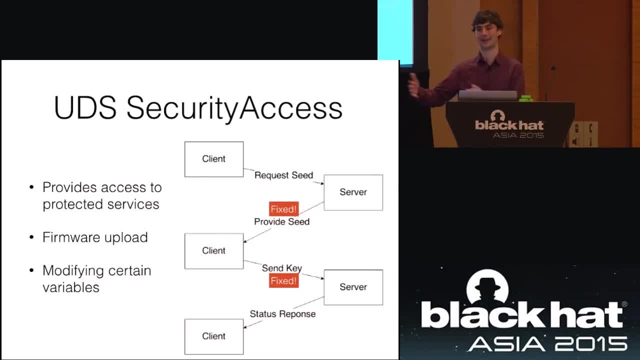 or while it's running through its end-of-line tests at the factory. you probably won't be able to see this happen, Though it's a good thing, Though some cars now are being updated over the air, So if you manage to log one of those, 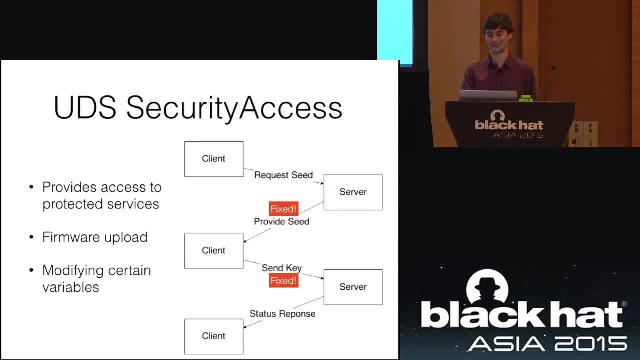 you could definitely be looking into this, But the thing that's really great about it is that both the seed and the key are 16 bits long, which means you can brute force the key space pretty quickly. They've sort of tried to stop you from doing this. 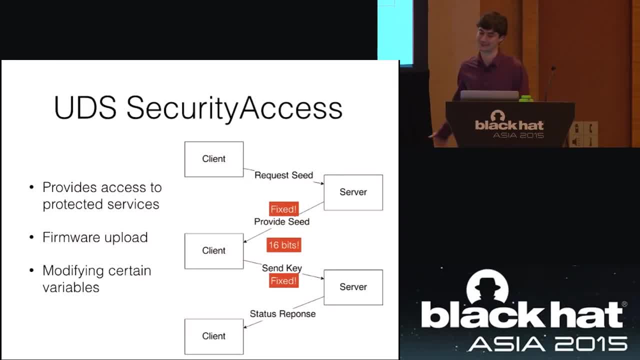 by putting in a delay, So you can't just send all the requests all at once. But it's not that long really. It's not something you can just jump in a car plug in and crack it, But if you have access to the car, 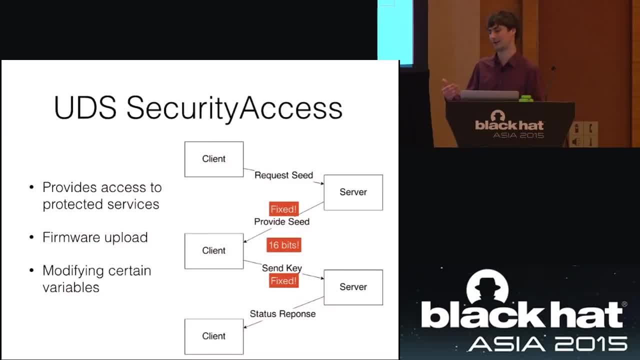 or if you've taken over a controller in a car. it's pretty much- maybe a couple days worst case- to get access to that. There was some research done by some folks at the University of Washington that they actually went into detail about how long these keys are. 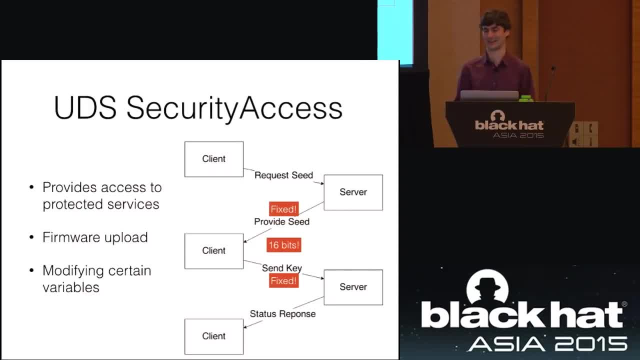 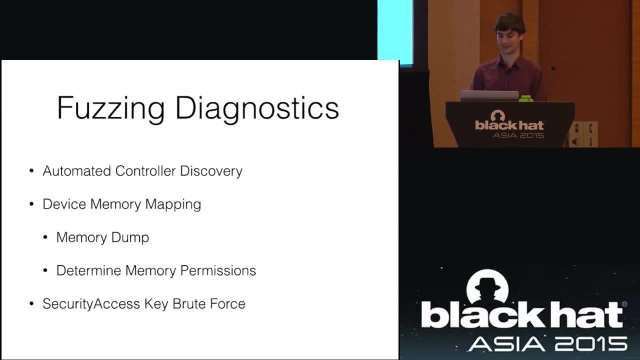 how long the delays are and figured out all the worst case times and said, eh, this is pretty bad. They're basically just assuming that you won't do. it is what they got out of that. So why might we want to look into these diagnostics? 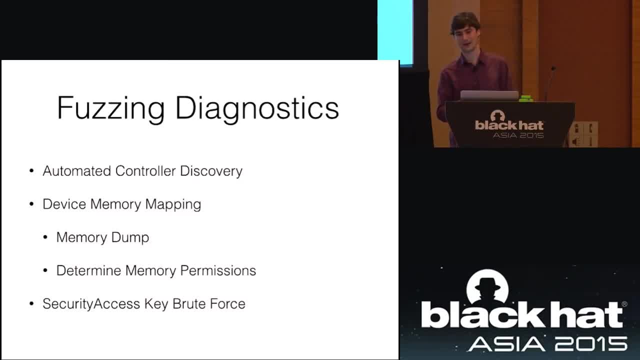 Well, fuzzing diagnostics, basically, can create a map of these controllers, right? So we did the automated controller discovery. That's a really simple example. But you can extend that example to automatically map all of the services provided by an automotive controller So you could plug in. 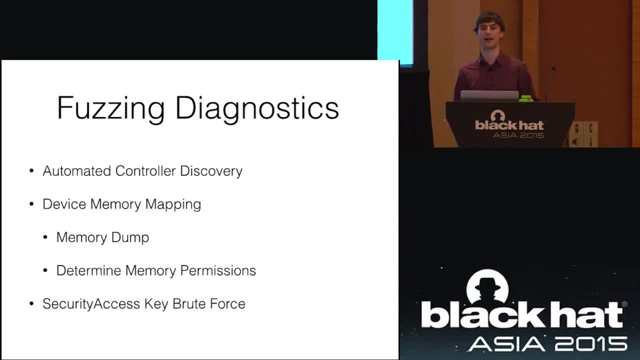 And just request every routine, every data identifier, every piece of memory You could request to do security access and figure out what all the different security access. They can have multiple levels of security access. You can get all of those And really create just a map of all the diagnostic features. 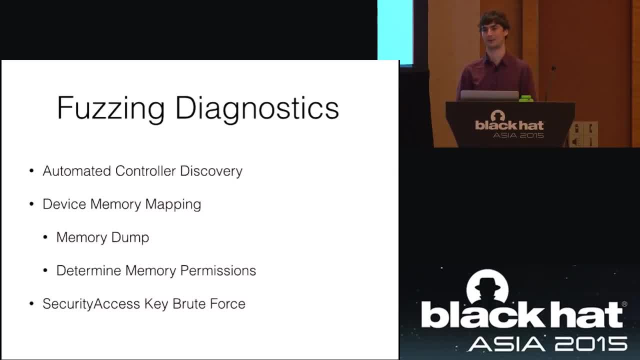 on the controller. And that's pretty much the starting point to playing around with this, Because once you know where you can look, you just start pulling stuff out. You can create memory maps, pretty much of a controller. You can take a look at where these values are. 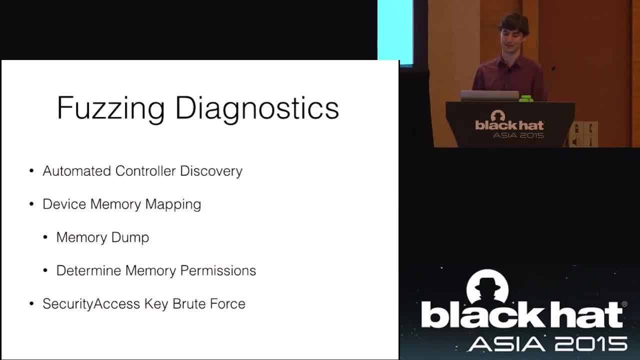 You can try to write things and figure out if you need security access And of course you can brute force that security access key if you so wish. So the concept of just fuzzing diagnostics I think is an interesting thing, Because the automotive manufacturers didn't really 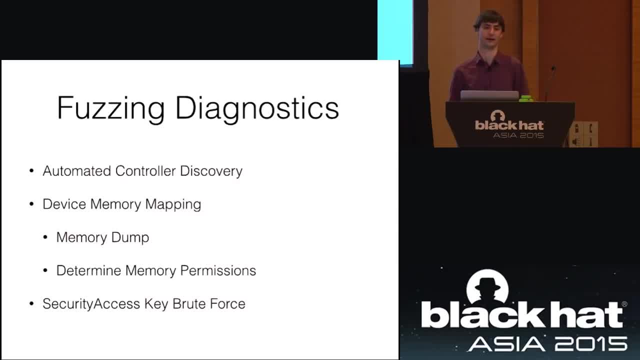 expect or didn't really care about people plugging into these buses. right, They designed the cars. They designed the cars in such a way that they figured: oh well, no one's going to play around with this, And as long as you can't remotely do it, 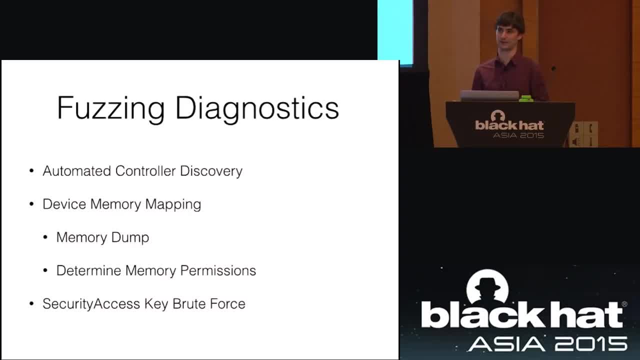 it shouldn't be a problem. So one side is: we're starting to see that as we connect cars to the internet, more you get attacks like the recent BMW one where, oh, they did authentication over HTTP And you could create a fake GSM base station. 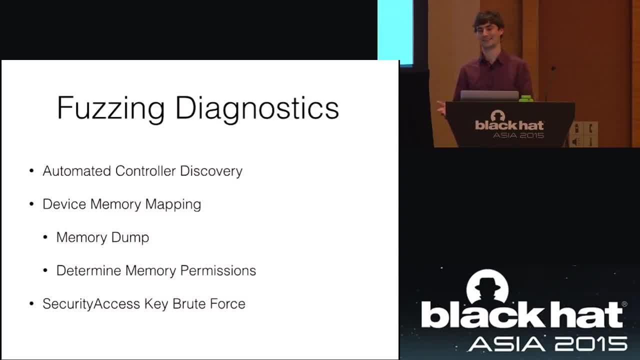 and man in the middle it. But the other side is that it lets people potentially get access to these CAN buses and exposes a whole bunch of functionality that the automotive folks just never really secured. So most of the stuff in automotive security is like: oh, it's just there and you can do it. 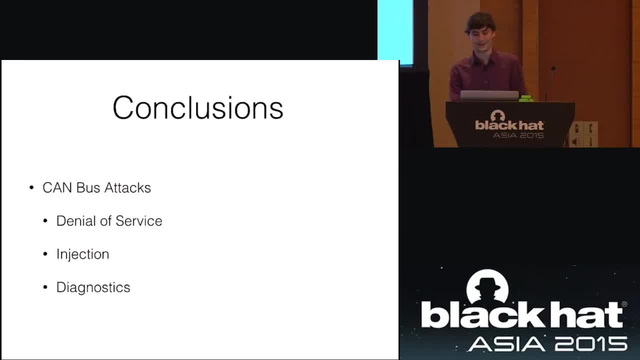 And the reason is because they just weren't expecting anyone to track. So just to conclude, here we talked about three different types of attacks that you can pull off. The first two are pretty simple: Just sending messages will let you do it. A denial of service, which is pretty easy, just spam zeros. An injection Injection attack, which it's really going to depend on what you're injecting. But you can fake out a lot of signals and just really confuse the vehicle in those cases. And then diagnostics, which is pretty much just a giant attack vector that hasn't been looked at in too much detail. 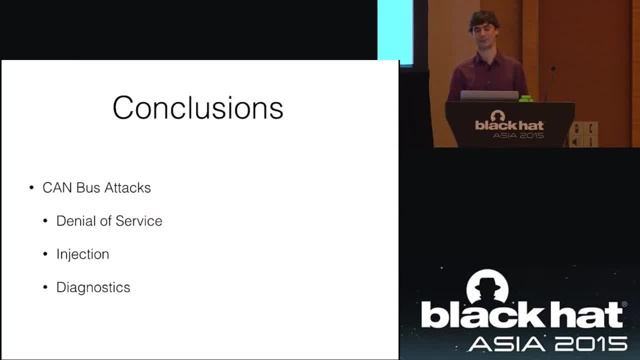 in most vehicles. But looking into the implementations, even if the implementations aren't bad, there's concerns. And then, once you go past that and look into problems where they've left behind little things, little things that were not implemented right, it could be even worse. 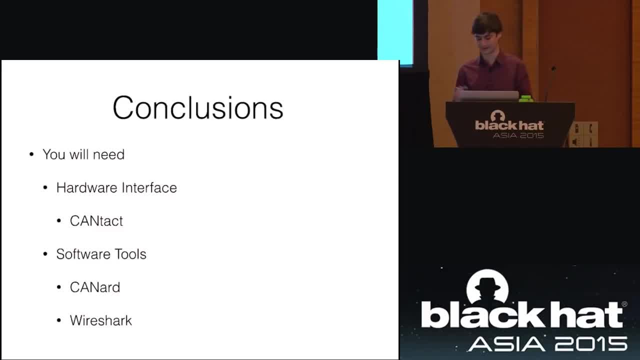 In order to play with this, you'll need a hardware interface. I mean, I've got to promote my own, I guess, which is this CanTac thing, This open source hardware tool for plugging into a CAN bus- And you'll need some software. 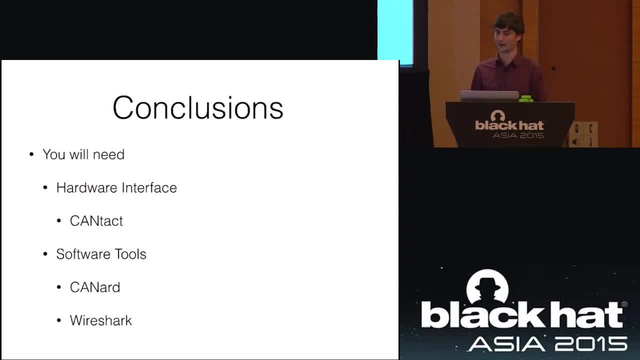 I like the Linux stuff, to be honest. Wireshark is great, This Kennard tool- it's getting better, I promise. But the idea is to make something where you can write scripts to play with cars and share them with people, so they can also play with cars. 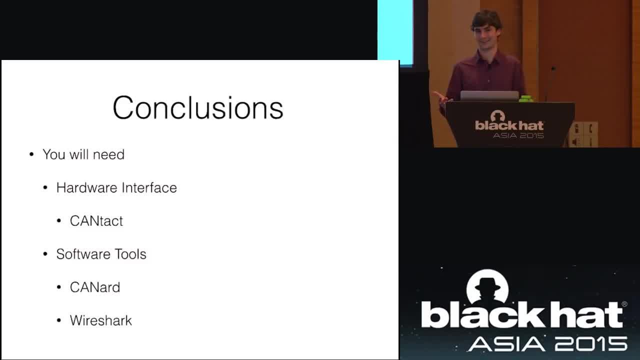 Because automotive security has been pretty much security through obscurity, to be honest, And now that we can start to look at it and make it easier to get on these systems, we can actually start to have some fun. So that's pretty much my main part of my talk here. 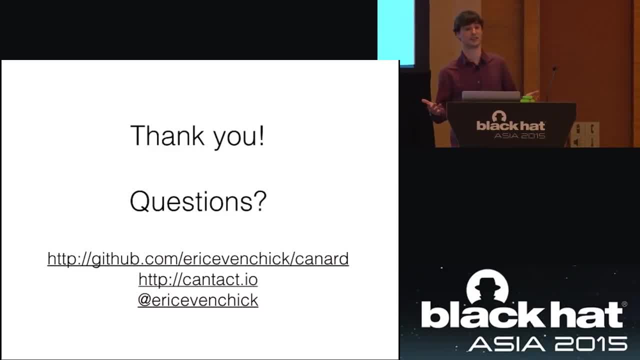 But I definitely want to move into questions about anything to do with cars, security and anything else you have on your mind. So over at the back there, OK. so the question was: do they share code for the implementations or do they write their own? 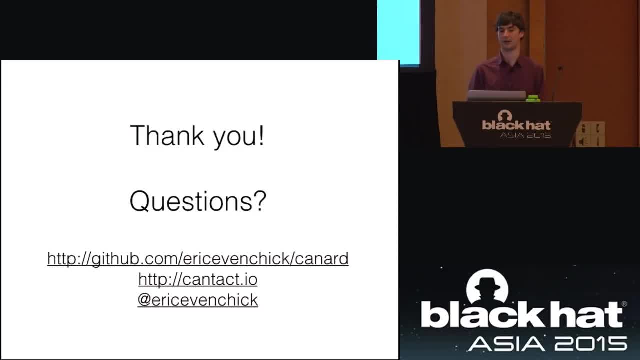 In a lot of cases they buy it from some vendors. Actually it's kind of fun to explain how automotive code gets written. So let's say you work in an automotive company as a software developer. You probably don't write any C or anything. that's in text. 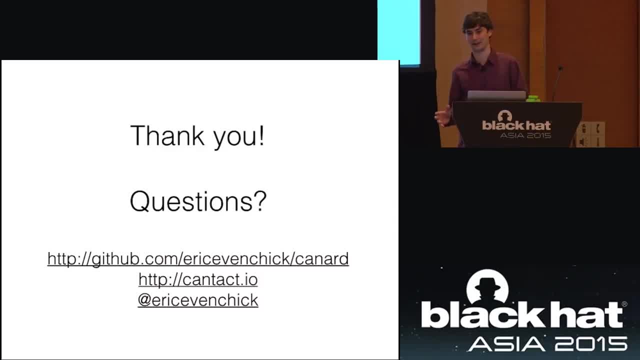 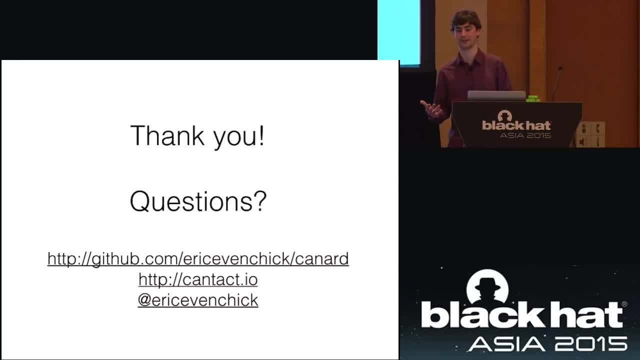 algorithms is done in Simulink, And if you're familiar with Simulink you'll know it's the graphical part of MATLAB, which literally is drag and drop blocks and connect them together with wires. That's how they develop these things. 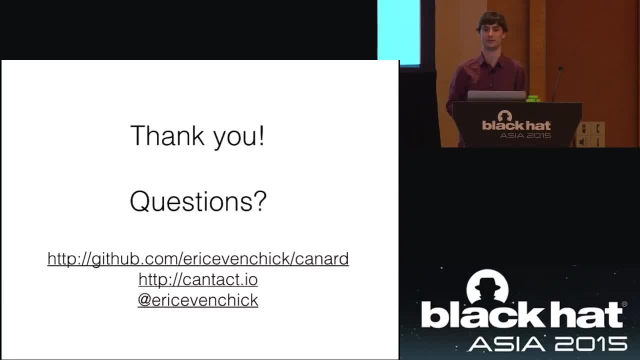 And that's what most of the people working in software positions at automotive companies do. Once they're done that, you prototype on a prototype controller. So I kid you not. you take your diagram, You hold Control, press B and out pops like an executable. 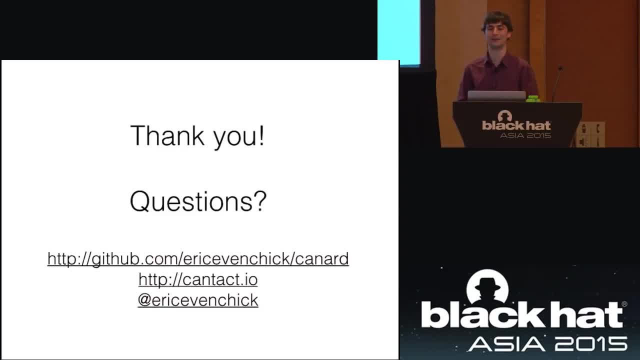 And you flash that to a controller and it usually works pretty well. Once they're done that development process, they'll work with an actual company that makes a production controller, like a Delphi or a Bosch or somebody, And working along with them they. 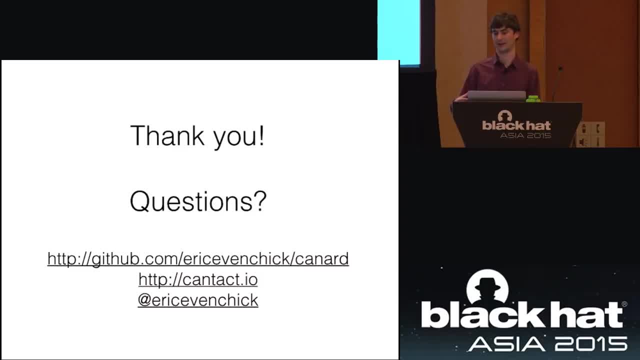 can actually get the cost down and get it into something they can put in the car. But all the code for things like CAN, things like the diagnostic stacks they typically buy from one of a few companies- probably the most common is Vector, who make the CAN tools as well. 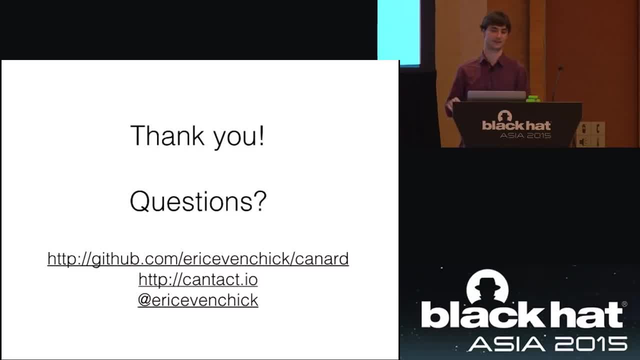 They sell stacks for UDS, They sell stacks for just generic CAN on different microcontrollers, all sorts of stuff. So the answer is yeah, a lot of it's shared But, even more concerning, a lot of it is cobbled together from different sources. 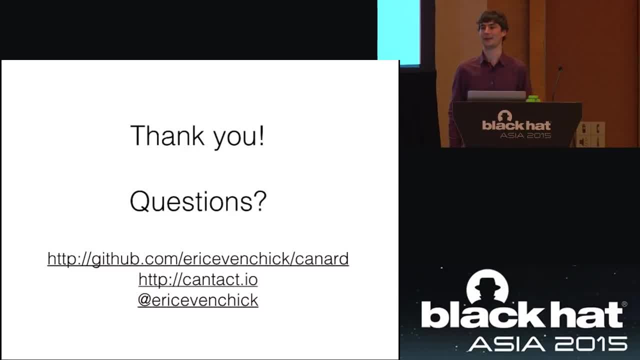 and then shipped Any other questions kicking around Here. I didn't see that one. Yeah, OK, the question was: how can you brick a car? Apparently, Charlie Miller managed to brick his car and posted about it on Twitter. 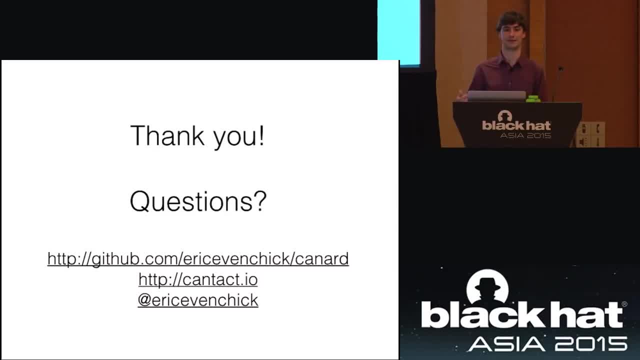 I'd say one of the biggest things is if it's a car that does have writable flash for firmware. Obviously, if you write some junk firmware to a controller, it's probably going to not end well. Other things you could do if you start messing around. 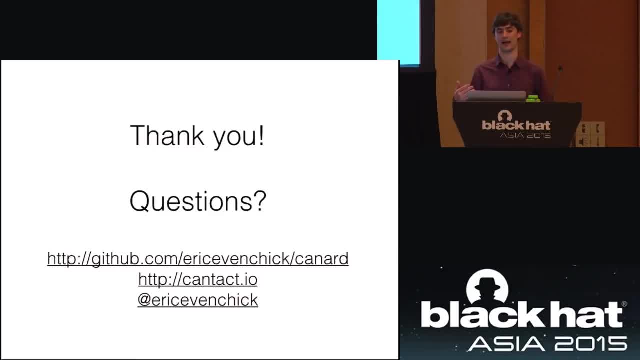 with VIN numbers. cars often have checks to make sure that all the VIN numbers and controllers match, So if you start playing around with that, you could potentially stop a car from starting. There's a few other checks that the car does. That stuff's really manufacturer-specific. 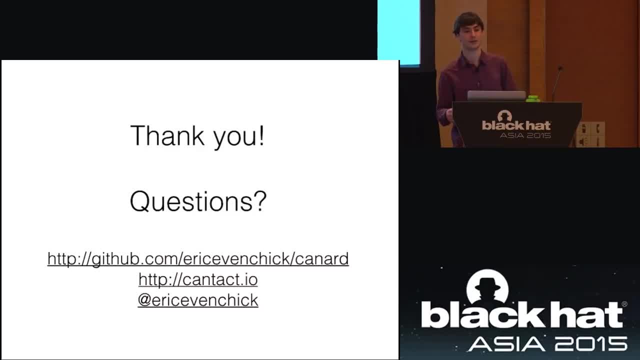 and they really don't like talking about it. But the immobilizer, so the thing that actually makes sure that you have a key, those use some weird challenge response stuff And you know If you mess with any of that, if you screw up. 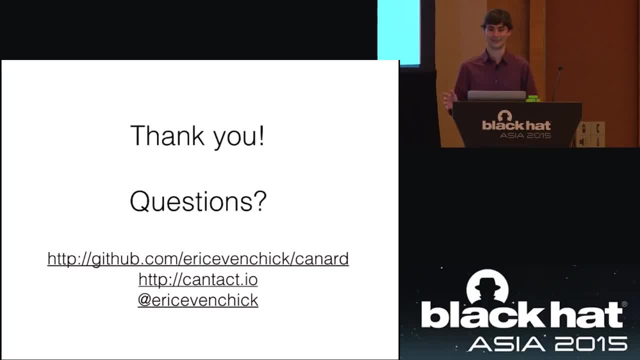 any of the seeds for that or anything, then the car will no longer do a proper immobilization unlock and then the car won't be able to start. So I think pretty much any of those. But the firmware one is probably like once you break the UDS code if it supports flashing. 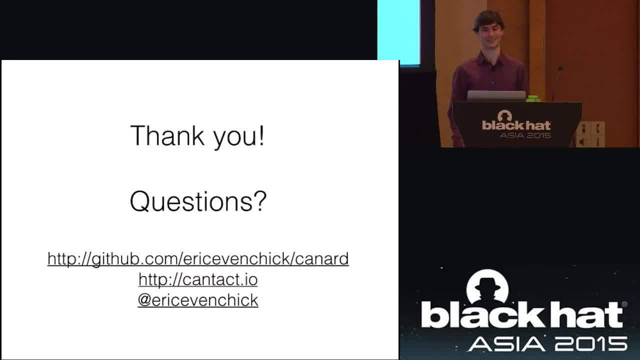 which quite a few controllers do. you can just write zeros to your firmware and that's definitely going to brick a car, Yep. So it sort of depends what level you want to do it at. You can fuzz like a raw CAN bus, which I didn't talk about too. 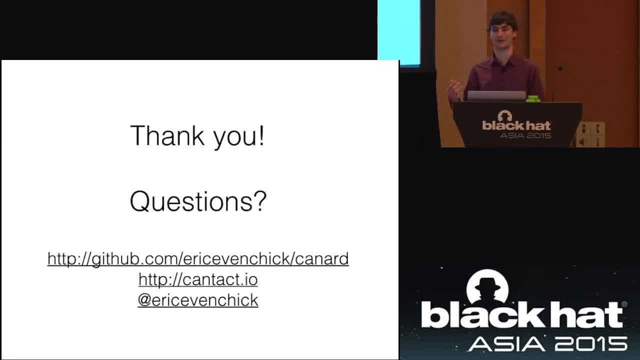 much, but if you're someone I was talking to today, I was doing that with planes, which sounds terrifying, But essentially you can send arbitrary data just in messages and kind of see what the responses were. So if you pick, OK, here's one great example. 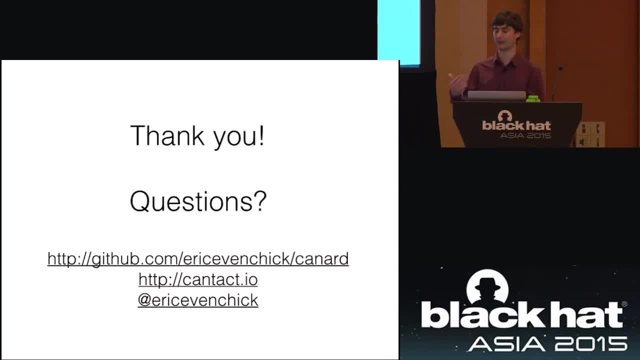 If you wanted to find where the message was that was controlling something like your vehicle speed or that was showing your vehicle speed, you could go through messages and send junk data until you manage- like randomly through messages, until you manage to get the expected vehicle speed. 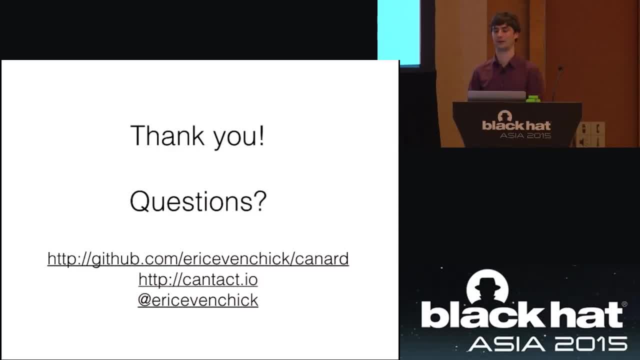 to show up on the display. So that's kind of the really low level of. you can fuzz raw like literally bytes. Then, going one level up, you can do fuzzing at the implementation level of the diagnostics. So in that case you can try one great example. 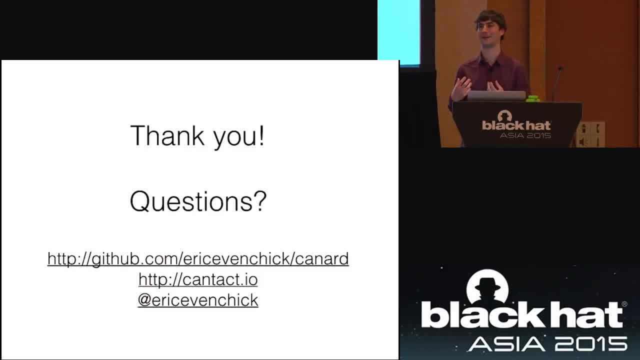 that I don't have the. I don't have the. I'm scared to do this on a real car- is: you can just ask it that routine control function. you can just ask it to run routine 0 through FFFF And it's going to do a lot of things. 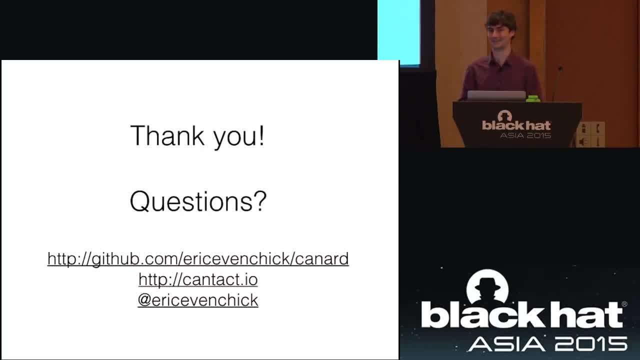 And who knows what it's going to do. The manufacturer does, But you don't. So by trying these things out, you can start to figure out what it is, And something like that is something you're going to want to do definitely. 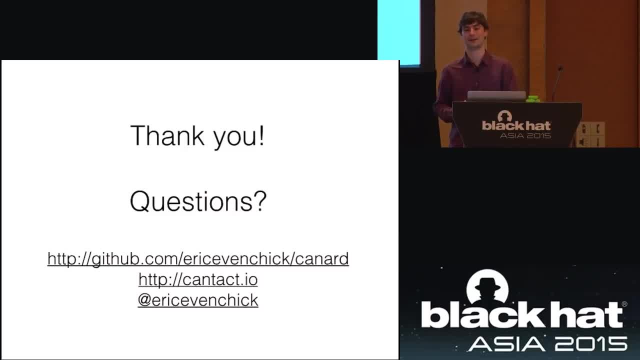 with the controller, on a bench, hopefully, and not in a car, But as you start to look at that, you can reverse engineer. what are these actions and what abilities does that give me? Oh, I got the. I'm not going to sell promotion, I'm sorry. 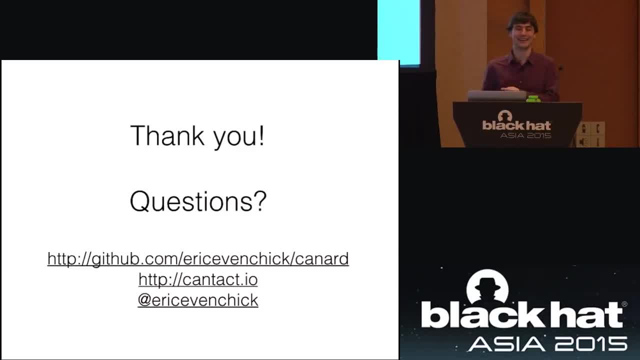 But there's a website there which is cantagio. There are a lot of things that you can do. There's like nine of them or something left from my. I did a first batch of them. There's not many left. If that ends up selling out, I guess I'll make more. 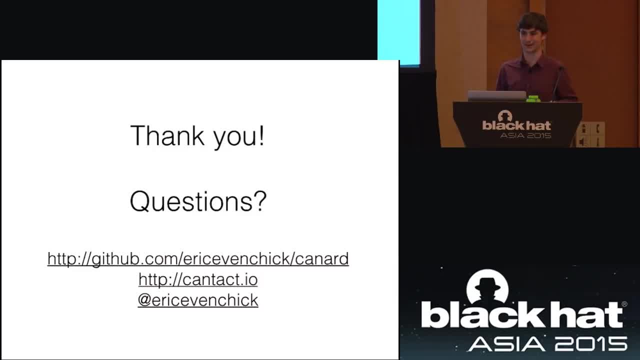 But yeah, it's kind of fun doing open source hardware for stuff like this, because a lot of this has been obscure and the tools were expensive And if I can make it cheaper to play with, that's kind of fun. Also, if you want to build your own. 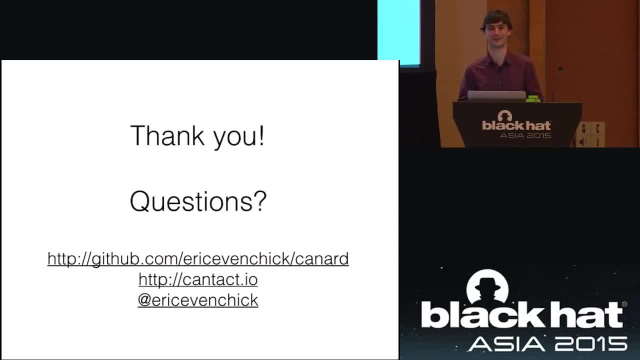 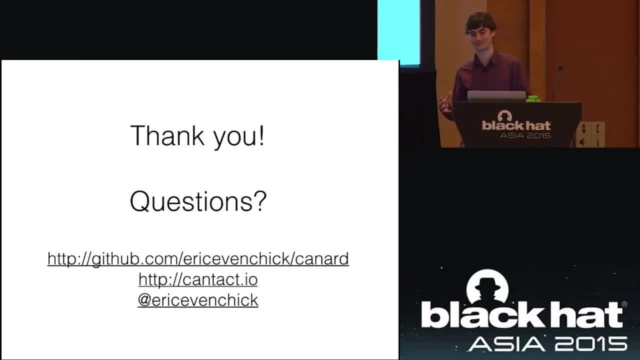 The real concern is, you know that's a controller that's potentially controlling an engine, And an engine is a very complex system nowadays, mostly because of emissions regulations. more than anything, An engine has things like variable valve timing that lets cams move around and slip. 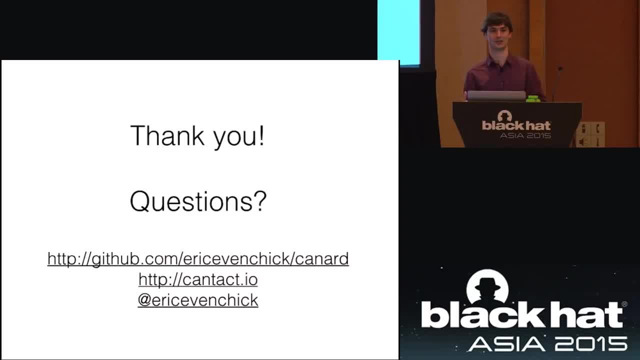 So you know, if you start fuzzing stuff and it's expecting a message that it's using to compute some of these, some of this stuff- message to compute something to do with how that engine's running- and you fuzz it, well, you could potentially cause. the engine to go into some terrible state. Now the engine controllers are typically pretty smart. They'll do a lot of sanity tests or checks on that data. They won't just let you destroy an engine. But in a real car it's probably not something you.